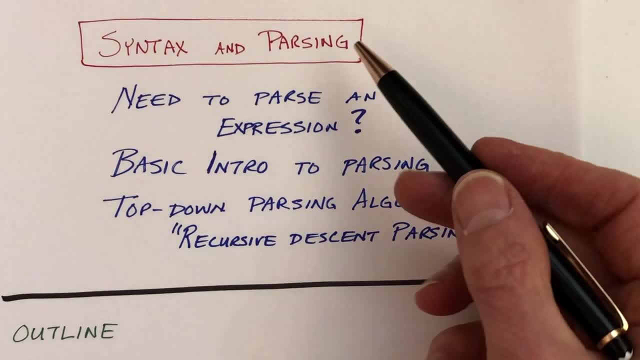 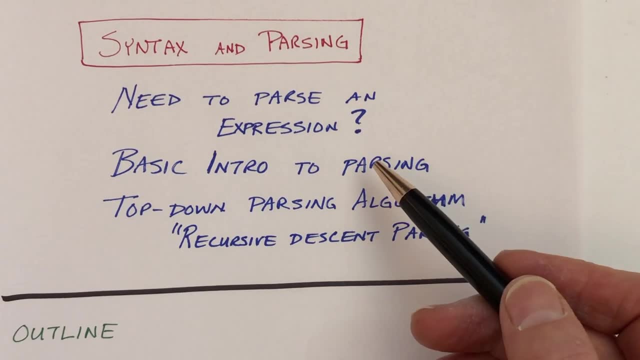 Hi, this is a brief tutorial on syntax and parsing. If you need to write code to parse an expression, this is the video for you. I'm just going to give you a basic introduction to parsing. It's a complex subject, but I'm going to tell. 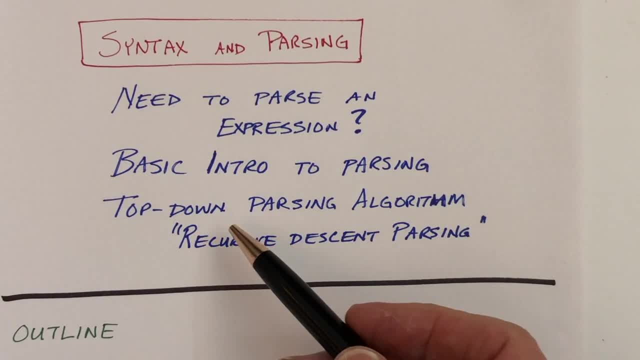 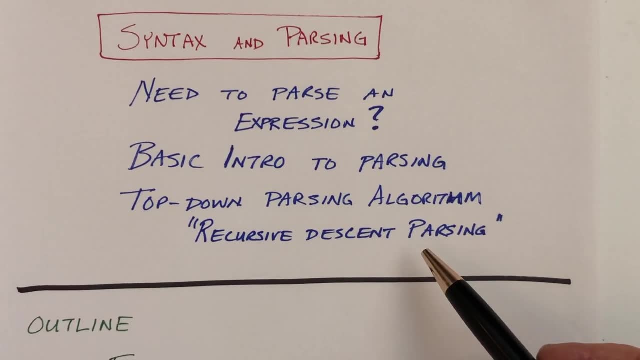 you all you need to know to get started. In particular, I'm going to talk about top-down parsing and I'm going to describe recursive descent parsing, which is the simplest algorithm and the only one you'll really ever need. So in this, 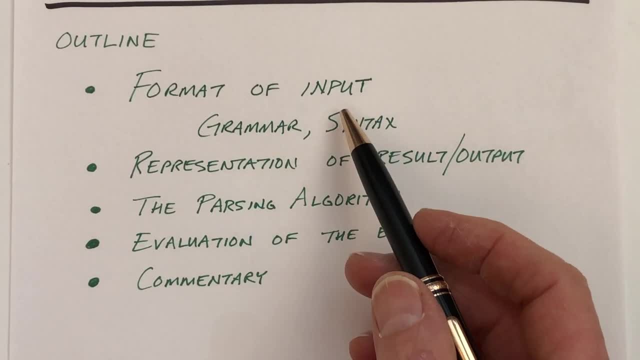 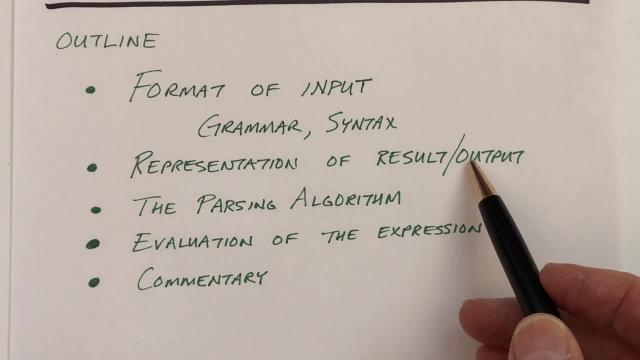 video. I'm going to start by talking about the format of the input, That is, I'll cover the ideas of grammar and syntax notation. I'll also talk about the output from the parsing algorithm, That is, how will we represent the result Then? 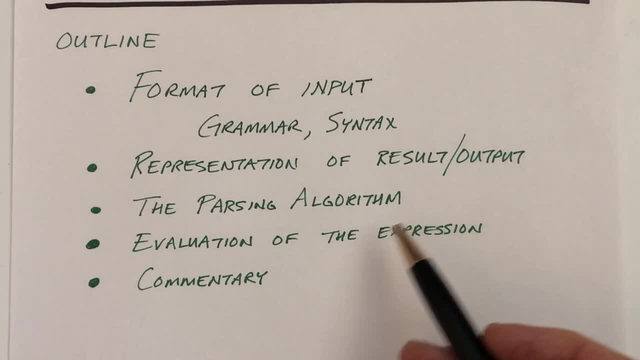 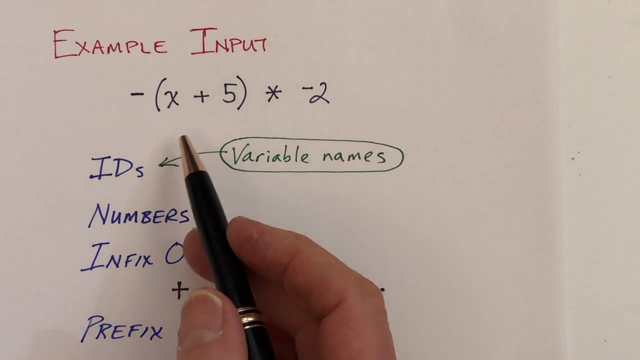 I will describe the recursive descent parsing algorithm And if you're parsing expressions, I'll also talk about how to evaluate the resulting expression. And finally, I'll close with some commentary. So our goal is to write code that will parse an arithmetic expression. Here's an example. 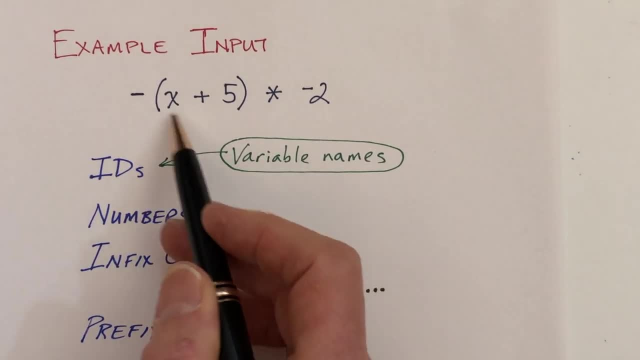 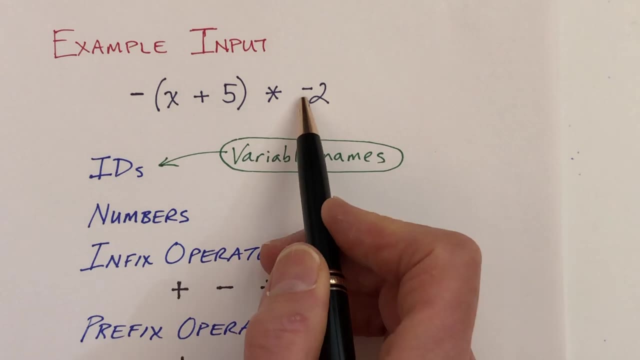 of the input we'd like to be able to handle. We see that it's got identifiers like X, it's got numbers, it's got infix operators that take two operands, it's got prefix operators like the negation, and we see parentheses. In addition, an. 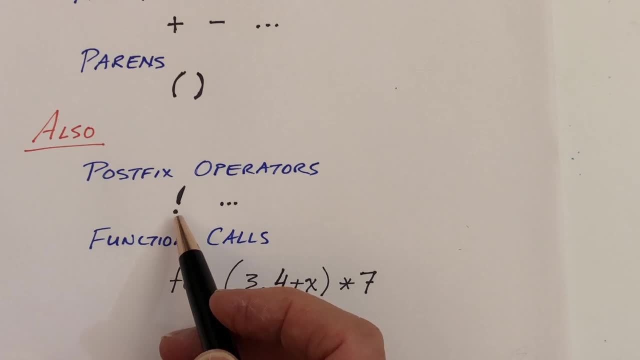 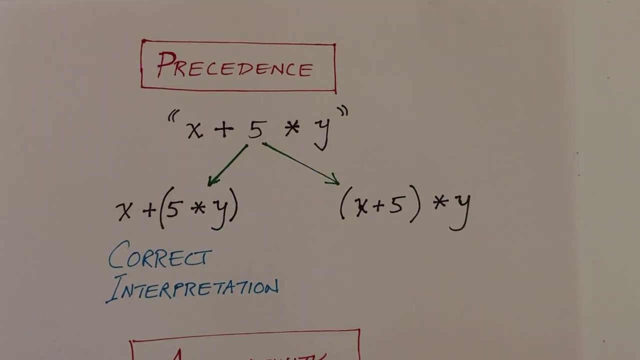 expression may also have postfixed operators, and factorial is the example of that, And it may have other things like function calls and so on, but these I'm not going to discuss. Before we go any further, I want to mention precedence and associativity. 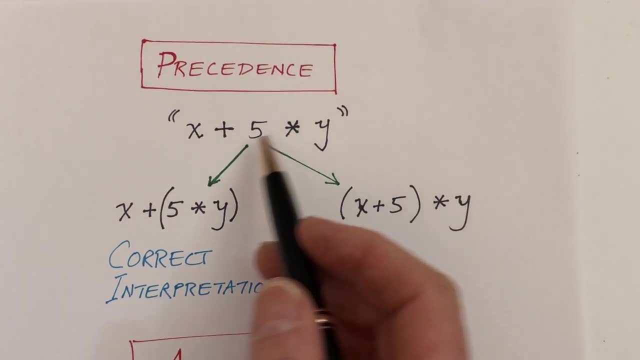 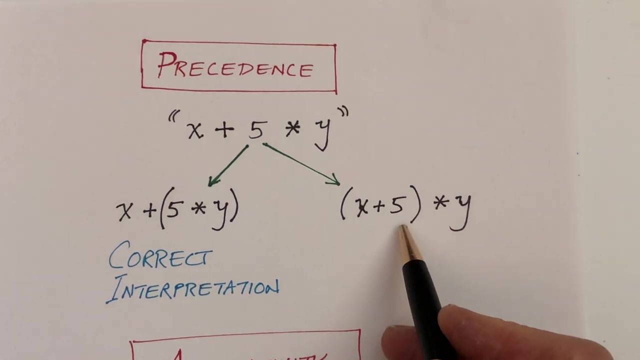 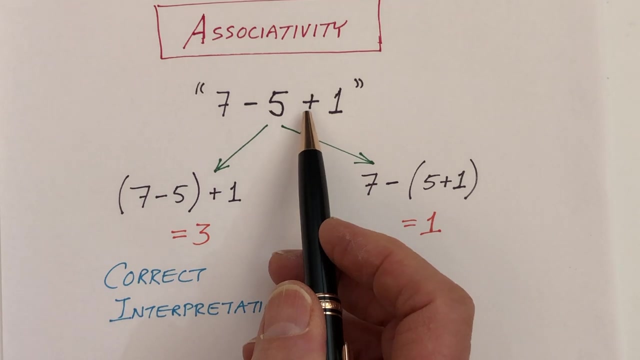 Remember that some operators have greater precedence. So, for example, this expression here should be interpreted this way and not this way. If the user of your parser intends to have this interpretation, then they had better add parentheses to the input to the parser With associativity. remember that with certain operators of equal precedence, like subtraction, 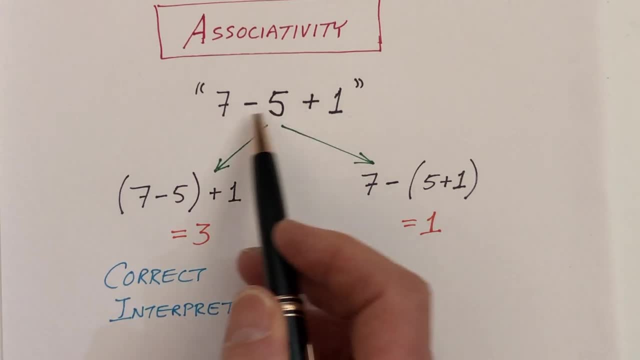 and addition. we want to process them in order, So this expression, for example, would be interpreted this way and not this way, which would give a different result. So our parser will need to take into account the proper precedence and associativity of 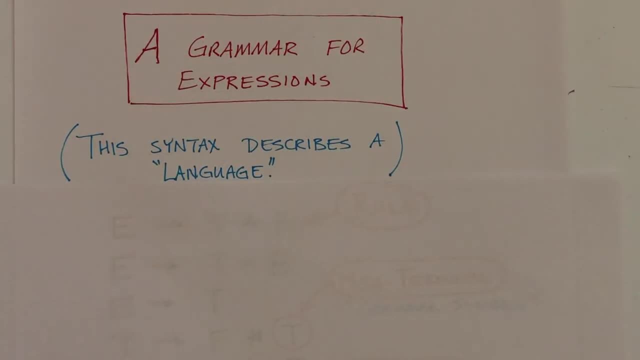 the expression and its operators. Before we can code up the parser, let's take a look at some other examples. To code up our parser, we need to describe exactly which expressions are to be accepted. That is, we need to describe the language of expressions that our parser will accept. 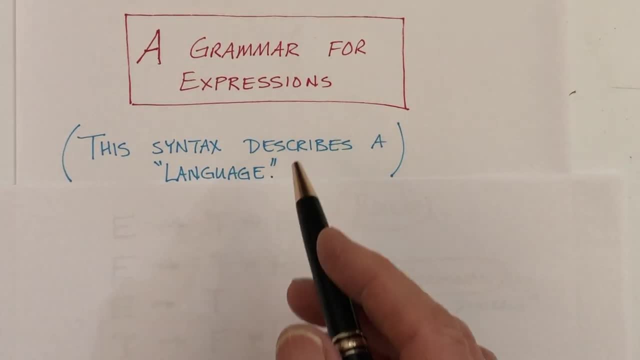 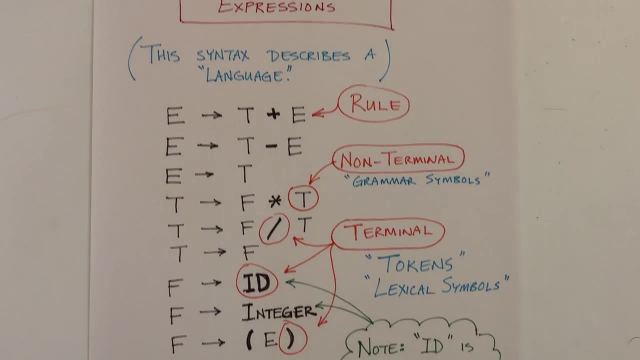 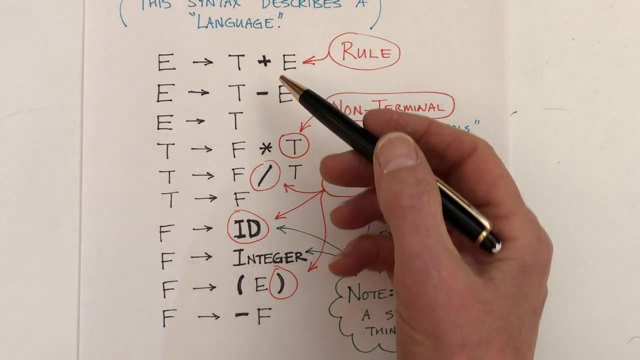 And to do that, we're going to provide a grammar for expressions. A grammar defines a language And here I have a simple grammar for expressions And let's go through it and take a look and see what we have. in every grammar We'll see a number of rules. 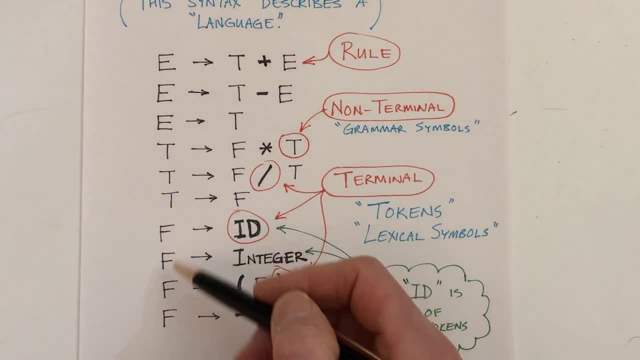 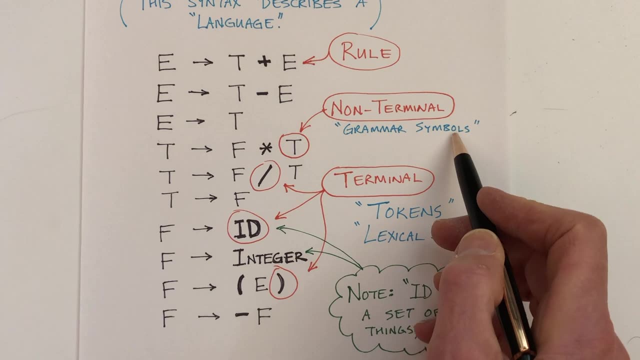 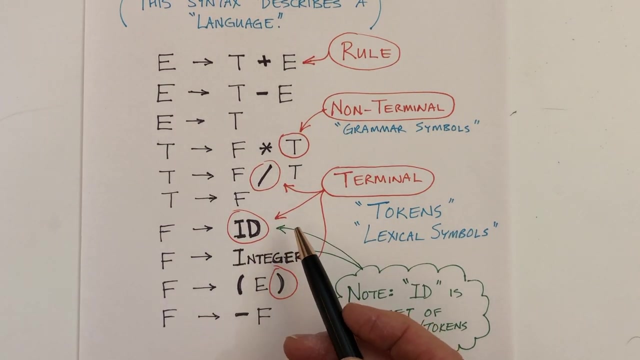 So here we see rules for E, rules for T and rules for F. These things- E, T and F- are called non-terminal symbols or grammar symbols, And this is the syntax for expressions. So these rules define exactly what it means to be a legal expression. 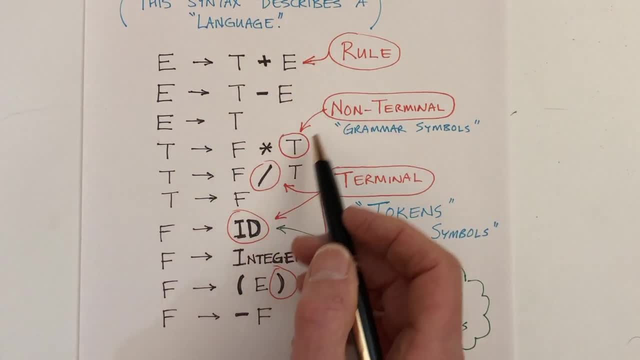 We also see in these rules on the right-hand side both non-terminal symbols like E, T and F, as well as terminal symbols, basically everything else. So we see plus, minus, the asterisk for multiplication, slash for divide. 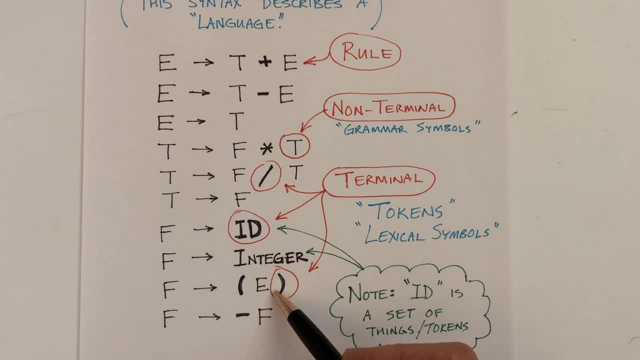 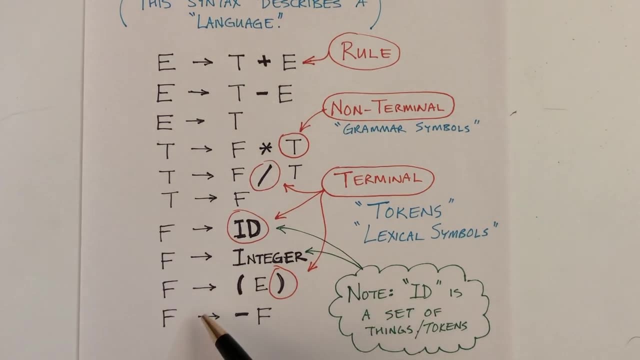 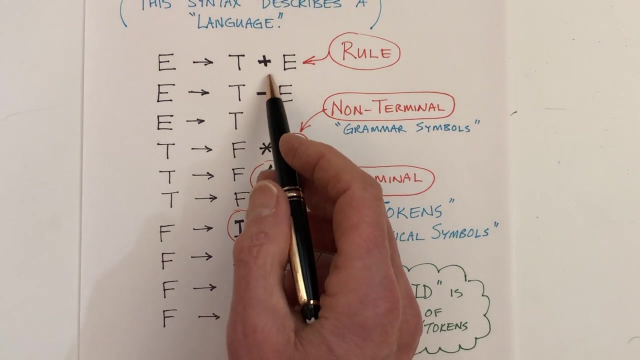 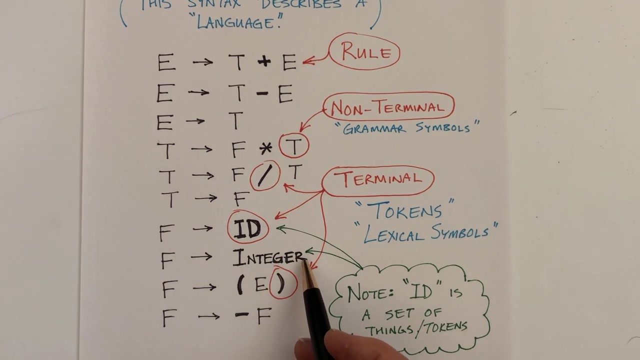 We see ID, integer and some parentheses. These are called the terminal symbols and they are not defined in the syntax for this particular grammar. Some of these, such as plus and minus, are literal things. they are just single characters. Others, like identifier and integer, stand for classes of inputs. 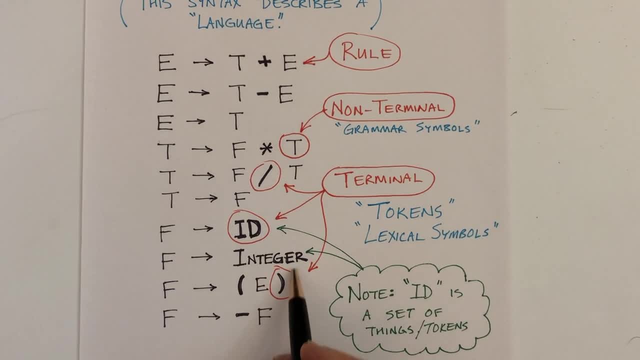 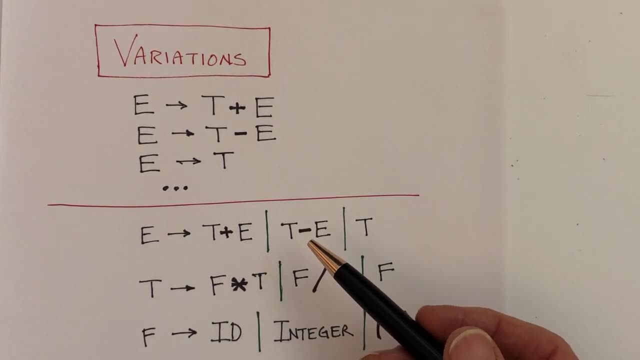 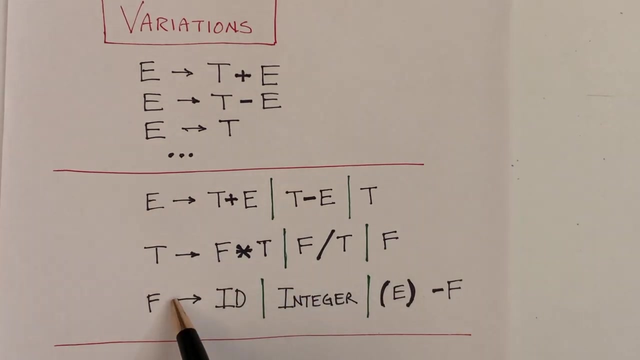 So there are many different identifiers, many different integers, There are some variations on grammar notation and I wanted to mention one important one. So here's our original grammar and we're showing the same exact grammar down here. We have three rules for E, but we're collapsing them. 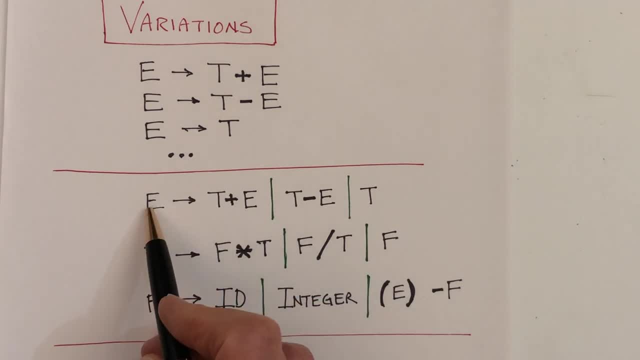 We're using a vertical bar to indicate OR, So an E, that is an expression, is either a term plus an expression or a term minus an expression or a term. By the way, E stands for expression, T stands for term and F stands for factor. 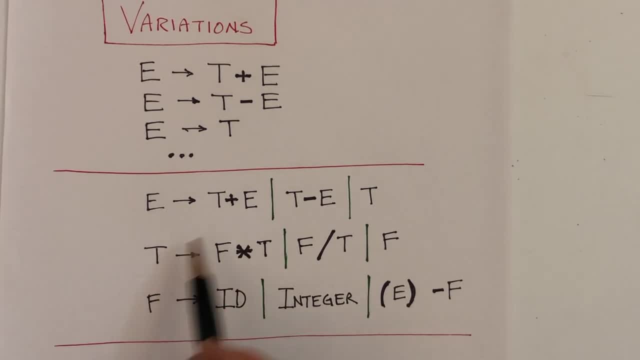 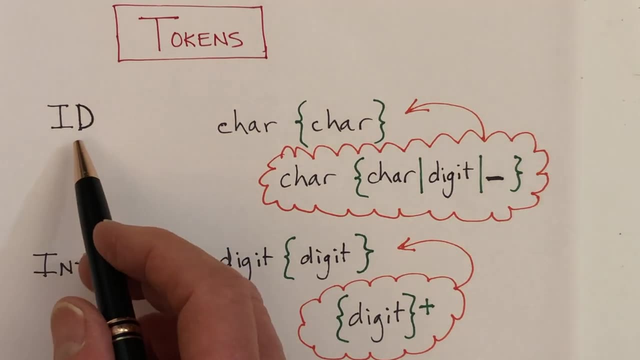 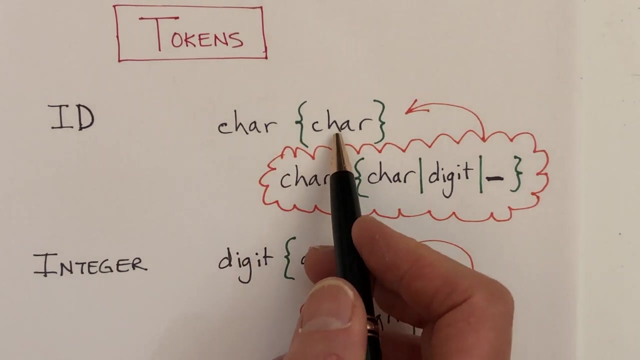 So if you multiply a bunch of factors together, you get a term. You add a bunch of terms together, you get an expression. For our purposes, we're going to define identifier as rule one or more characters, So this notation here means one character followed by zero or more. 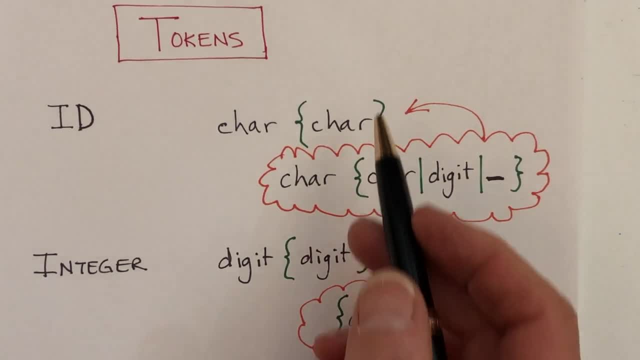 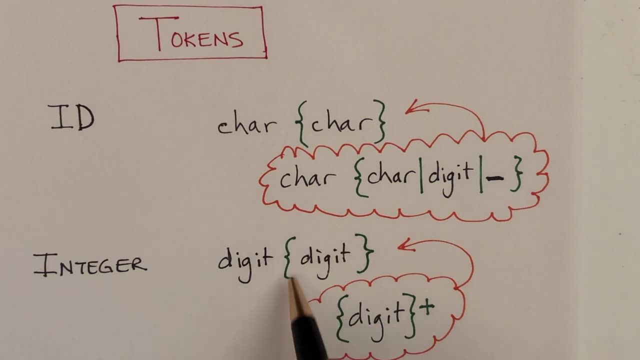 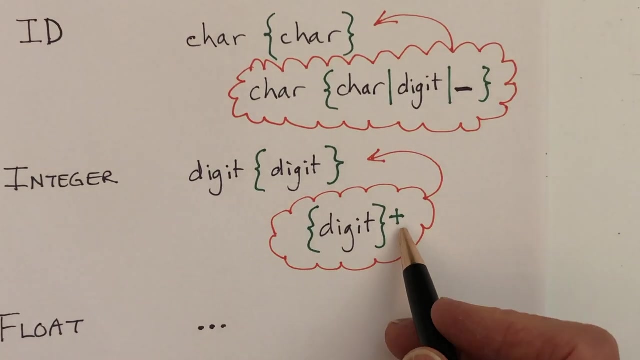 characters. The braces mean zero or more. We'll define integers as one or more digits. So again you have the curly braces. Another notation you might see is curly braces with a plus sign and that means one or more occurrences. So these two are equivalent. 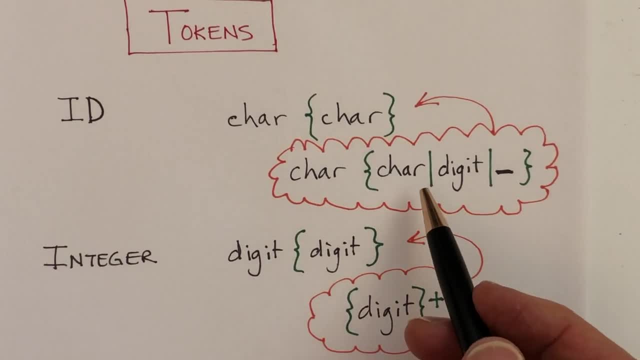 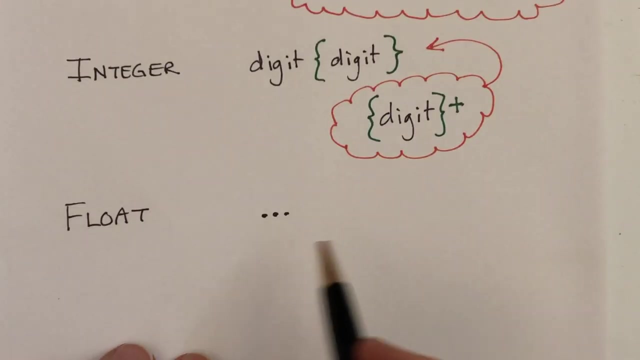 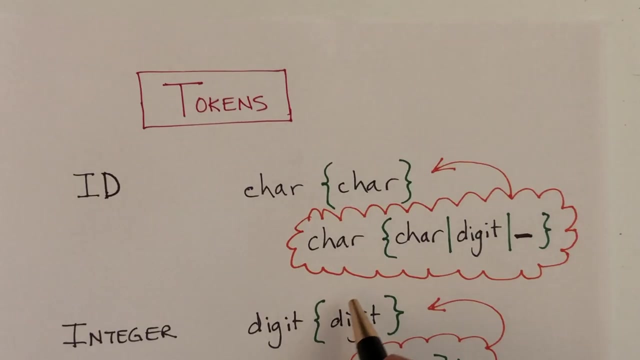 Many programming languages have slightly more complex definitions for identifiers. For example, we might define identifiers as a single character followed by zero or more characters, digits or underscore characters. A programming language might also define tokens like floating point numbers and so on, but we won't go into that here. When we scan one particular identifier, 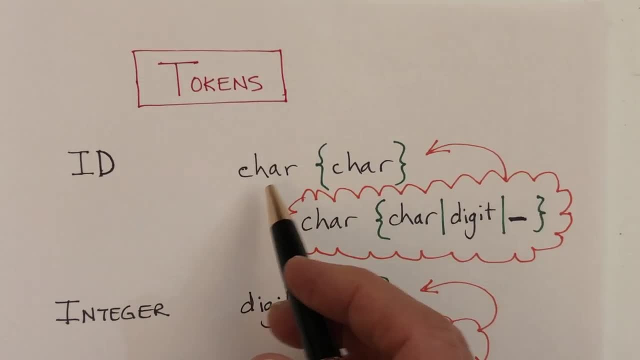 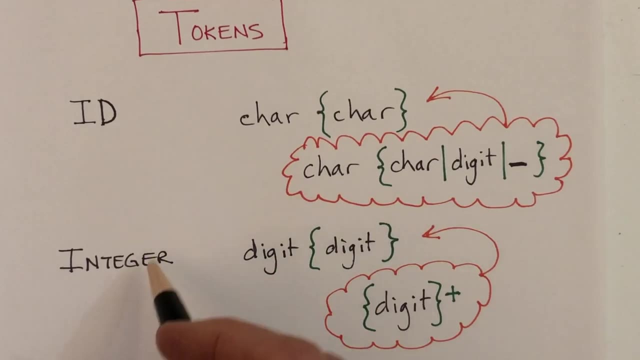 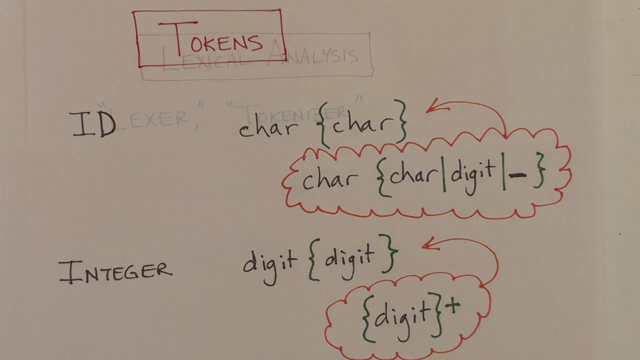 that will be a token. So our input consists of a series of tokens. The token could be an identifier, It could be a plus symbol, or a multiplication symbol, or a parenthesis, an integer and so on and so forth. So we'll view the input as a sequence of tokens. Before we can parse the input, we need to. 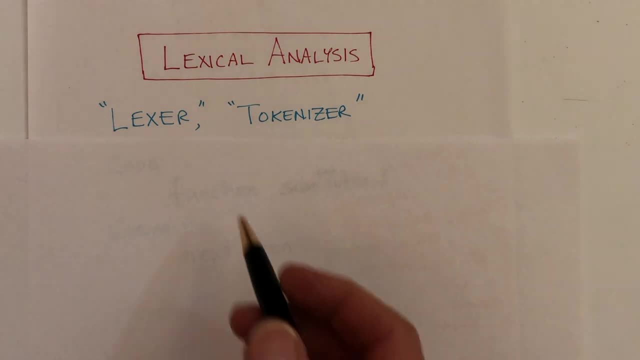 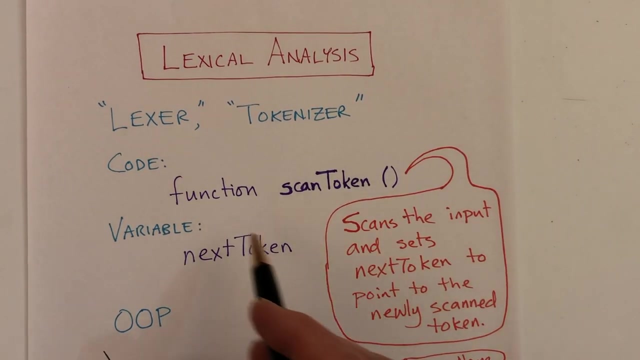 break it up into a sequence of tokens. This is known as the lexical analysis part of your parser. And we have a lexer, sometimes called a tokenizer, that performs this tokenization of the input, So it'll read the input and break it into tokens. So in our organization, 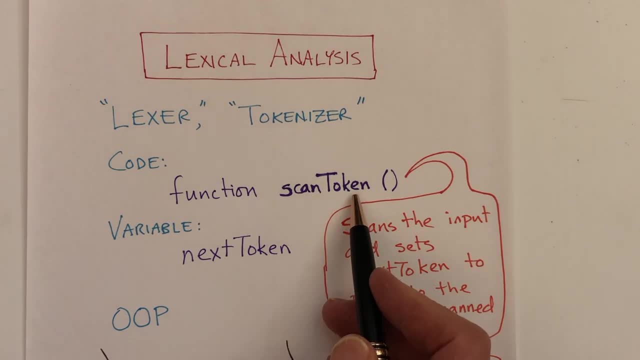 we will assume that we have a function called scanToken. I'm not going to specify it here, but we'll assume that it scans the input, reads in from the input and we've got a variable called nextToken And every time we call scanToken it will set this variable to point to the newly. 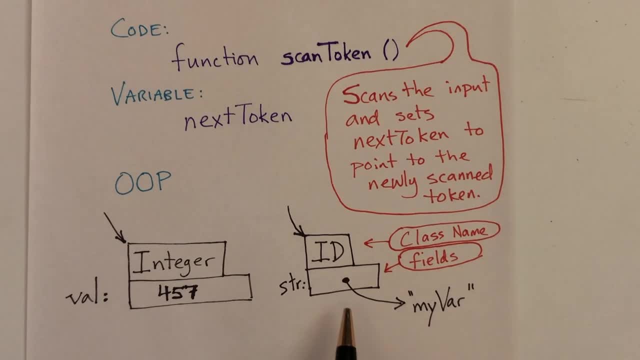 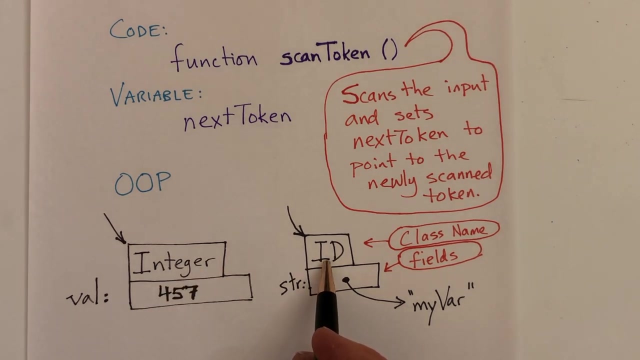 scanned token. I'm going to assume that we're using an object-oriented programming language, and so we'll represent tokens with objects. So here's an object of class Integer and here's an object of class Identifier. I show my objects this way and the class Integer has: 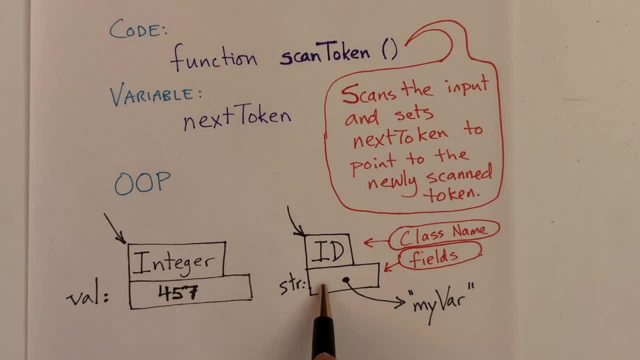 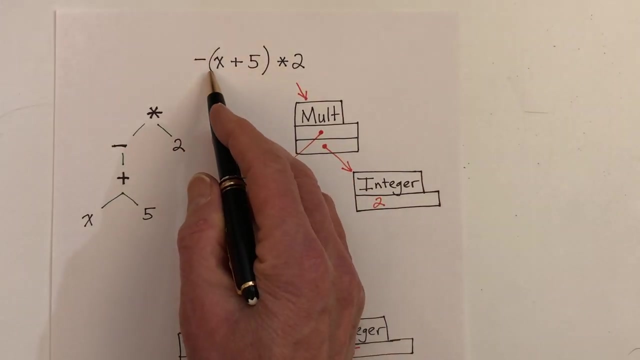 a single field value and the class Identifier has a single field called string, which points to, to the actual characters that are involved in the identifier. The goal of our parser is to read in some expression such as this one right here and produce some output, so some representation of the expression. 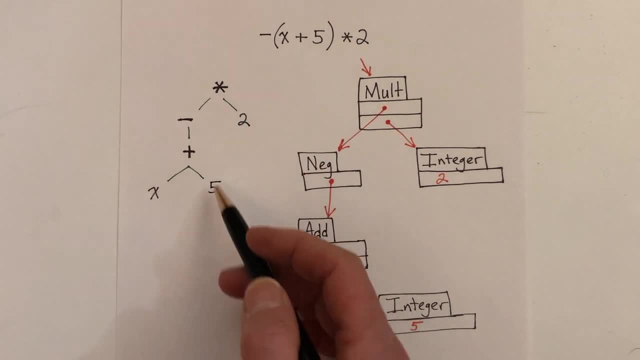 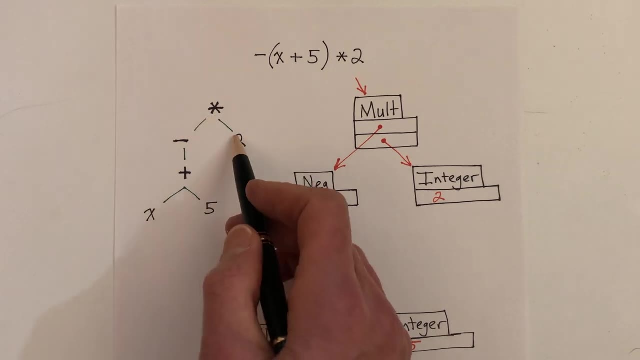 So the first representation of this expression is shown right here, and this is the simplest. You can see that we add x and 5 first and then negate that, and then we multiply that with 2. So this is the first representation of the expression and this is the second representation of the. 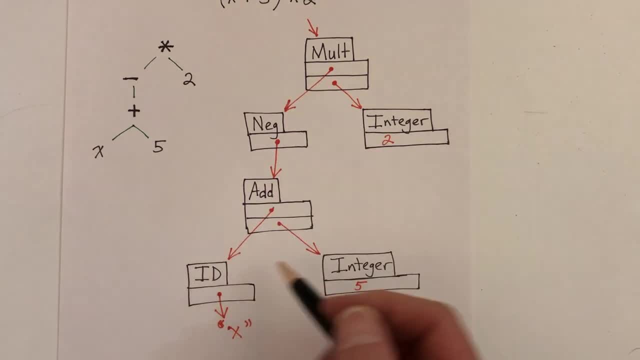 expression. and this is the third representation of the expression and this is the fourth representation of the expression. So we'll represent the tree with objects in a pretty much straightforward, one-to-one way. We'll have classes called multiply, negate, add, subtract and so on. 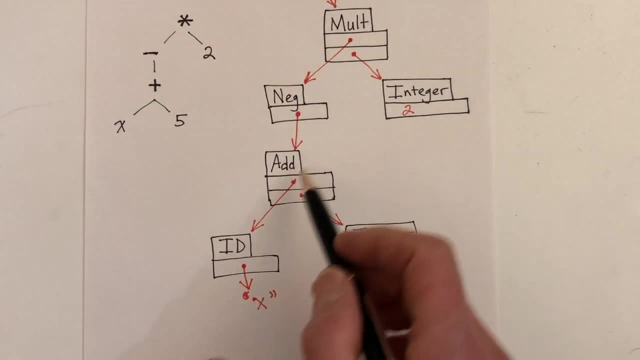 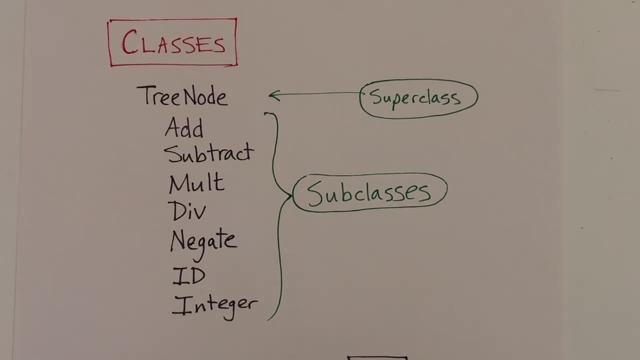 as well as classes for identifier and integer. So this tree right here is naturally represented with this collection of objects. We're going to use these classes here. So we've got a class called add, subtract, multiply, divide, negate, identifier and integer. We'll also have a class called tree node. 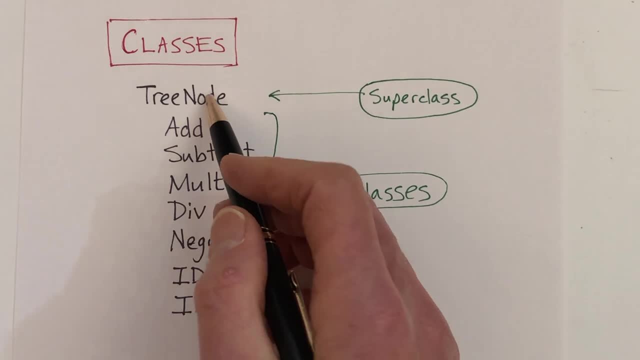 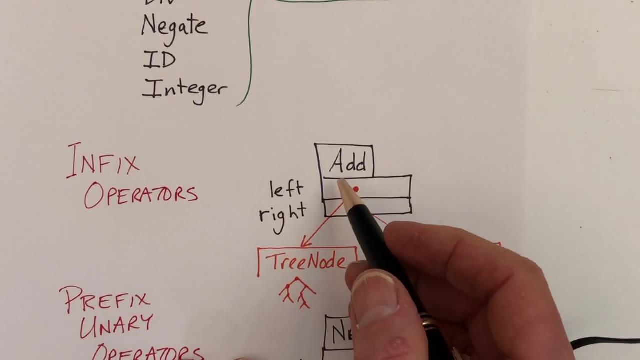 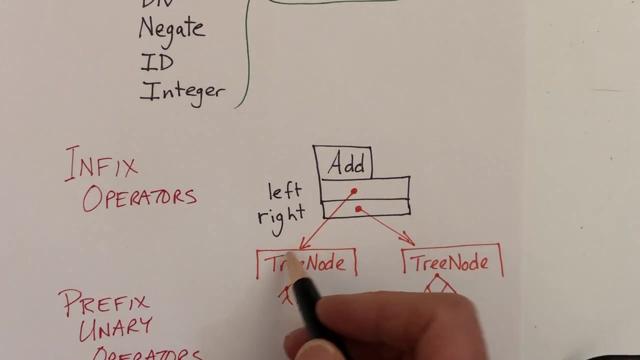 and all these others will be subclasses of that superclass. So these are all different kinds of tree nodes. So for the infix operators like add and multiply, we'll have two fields in the class. One is called left and right, and these will contain pointers to other tree nodes. 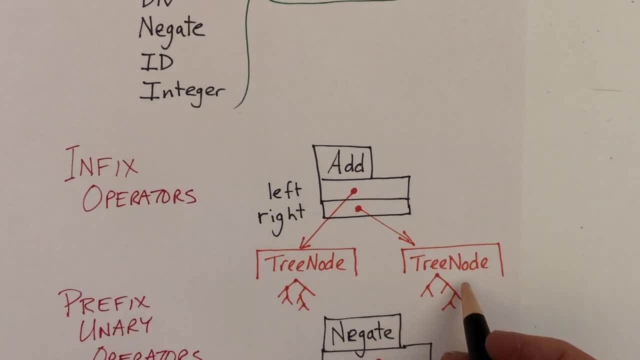 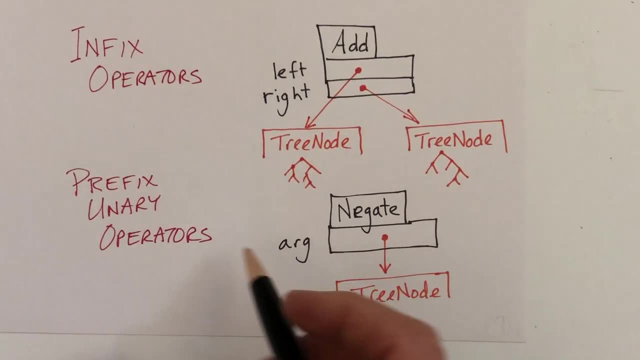 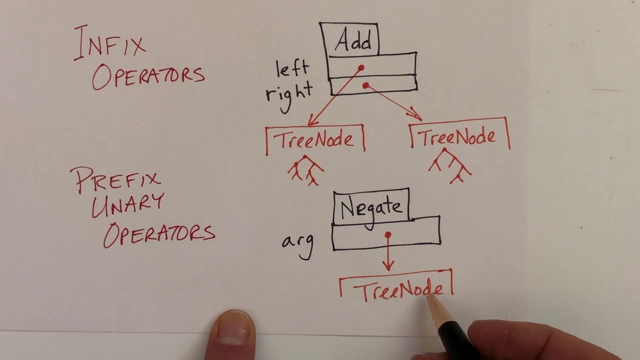 depending on what kind of sub-expressions are being added together. Well, that will determine what exactly is down here being pointed to. For prefix operators like negate, we'll have just a single field called arg or argument, and that will point to some tree node. 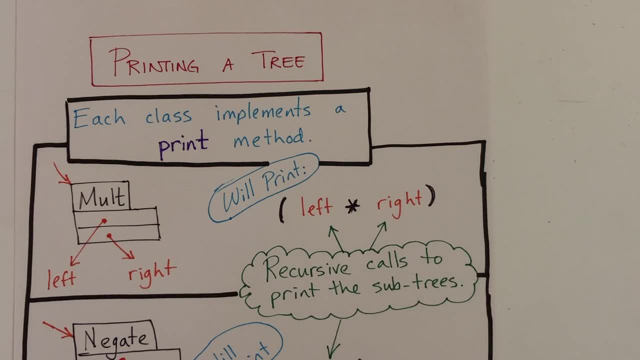 You're probably going to want to have some way to print out an expression If, for no other reason, you'd like to verify that your parser is working correctly by printing out the internal representation that the parser is producing. So let's suggest that we have a print. 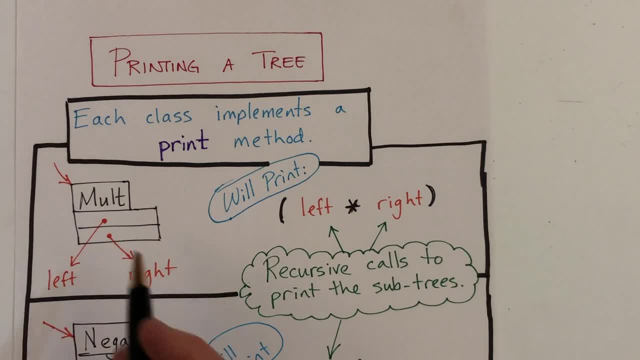 method for each one of our classes. These are going to be recursive methods that call each other, So, for example, the class multiply or any other infix operator would work like this: It's got a pointer to the left subtree and a pointer to the right subtree. 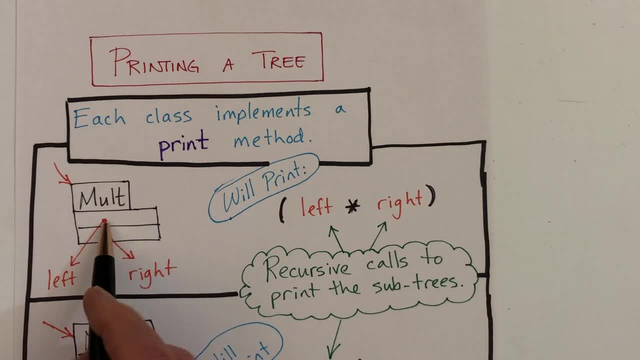 So what print is going to do when called on this particular node is print an opening parenthesis, then it's going to call itself recursively to print out whatever is pointed to by the left pointer, then an asterisk, then call itself again recursively to print out. 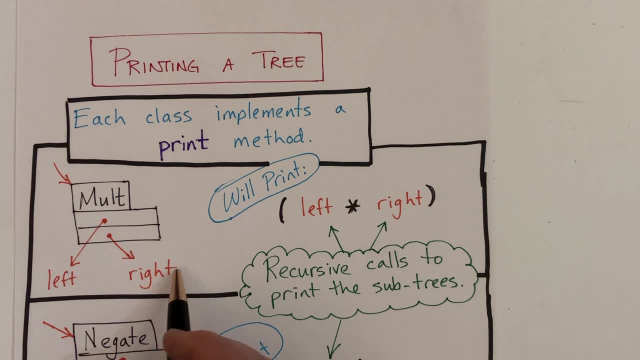 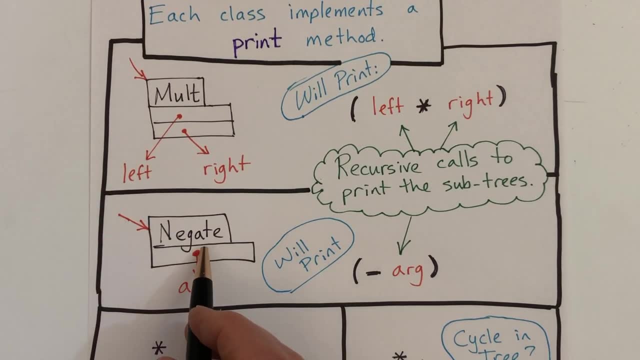 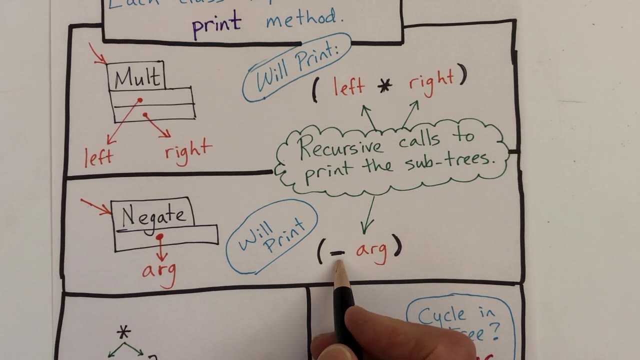 whatever is pointed to by the right field and, finally, a closing parenthesis. A unary operator like the negate class just has a single field pointing to its argument and it will print an opening parenthesis followed by the negate symbol, followed by the subtree. 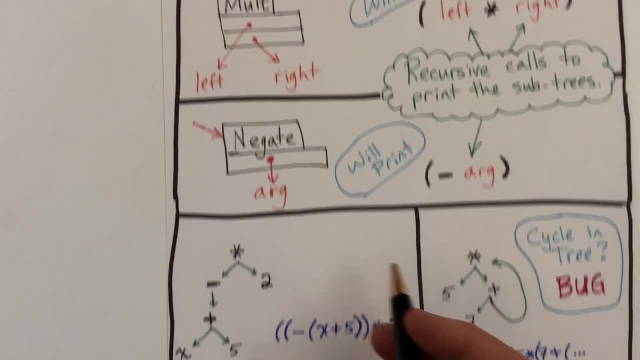 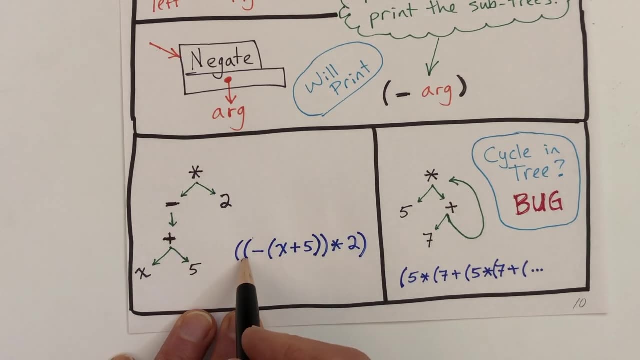 whatever it is, and then a closing parenthesis. So, for example, if you have this particular expression, it's going to print out something like this: You'll see it's got a lot of parentheses, but that makes sure that the output is exactly unambiguous, So you can be sure exactly. 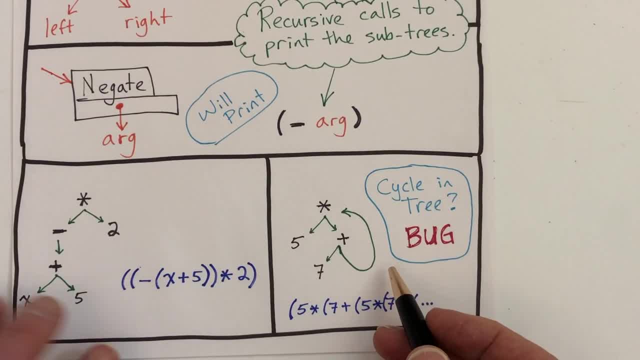 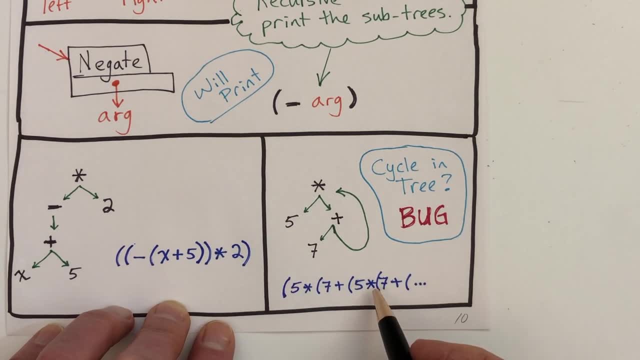 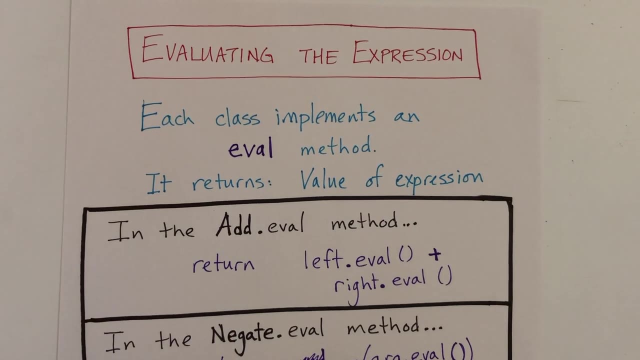 your representation is. I should mention that if, for some reason, you get a cycle in your tree and you try to print this out, you run into an infinite loop. You just keep printing five times seven plus and so on. Let's assume that your parser has read in an expression and built an. 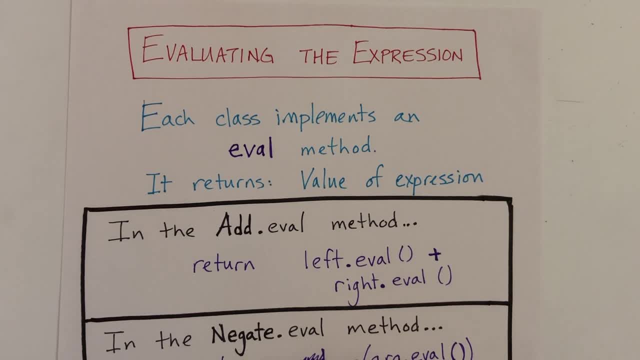 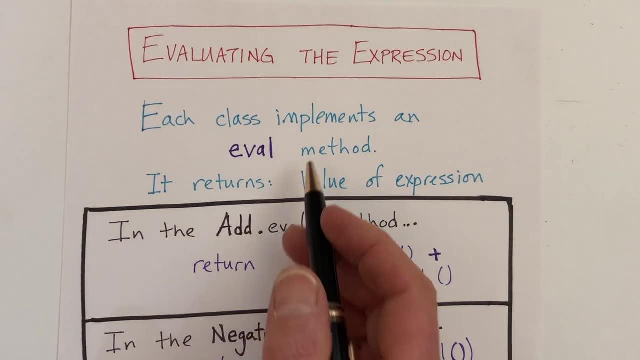 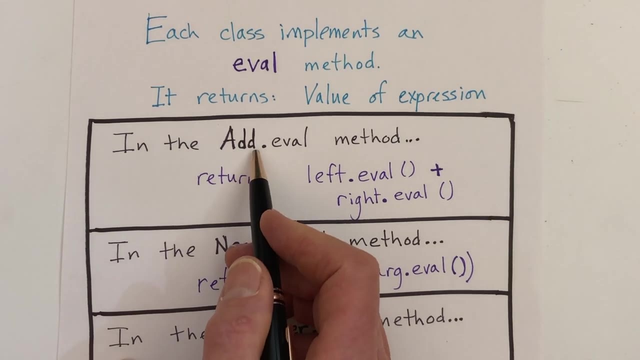 internal representation of that expression. Now you'd like to evaluate the expression, So for that, I'm going to go ahead and show you how to do that. I'm going to go ahead and show you how to do that. So, for example, in the add class we've got an eval method that simply calls itself recursively. 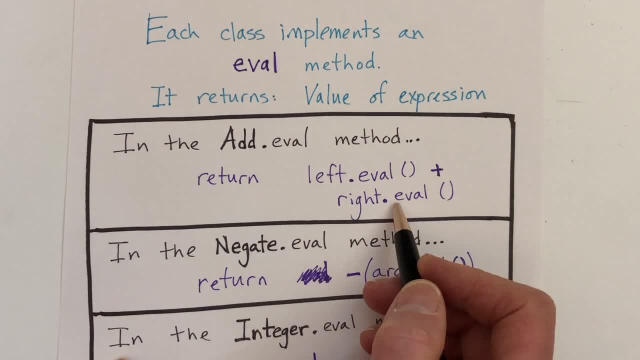 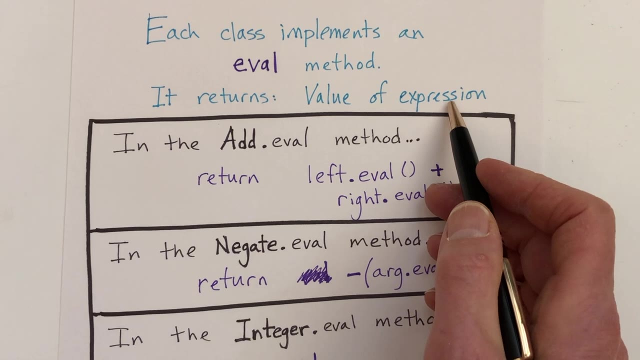 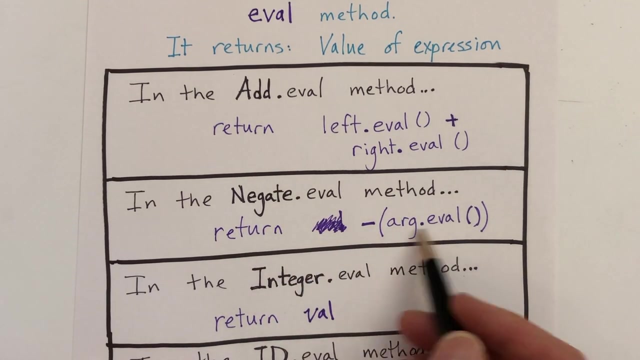 on the left subtree, then calls itself recursively on the right subtree, adds them together and returns the result. So each one of these eval methods is going to evaluate the subtrees and then return the final value of that complete expression. A unary operator like negate, would simply call itself recursively on. 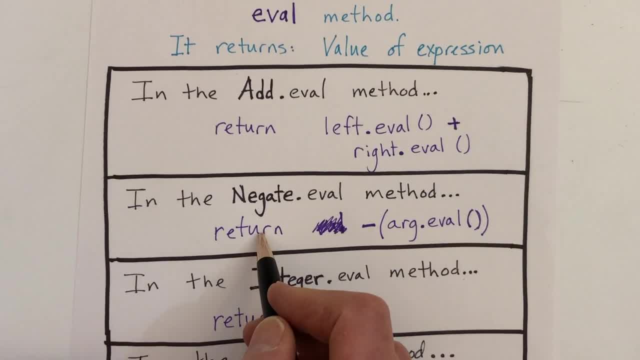 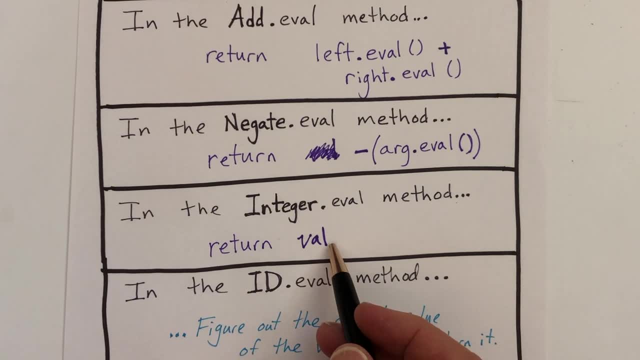 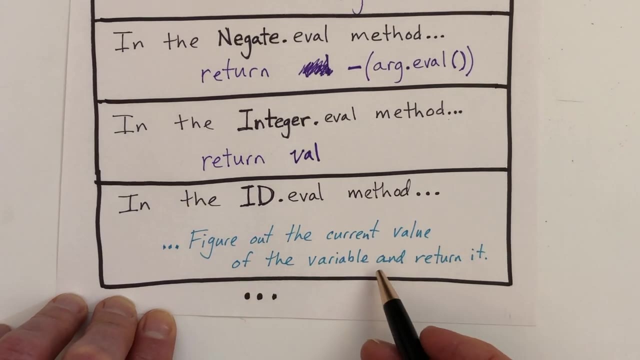 the subtree, negate that and return the resulting value. If the node happens to be an integer, then the eval method simply returns its value. If the node is an identifier, then well, we have to figure out what the current value of that variable is. and 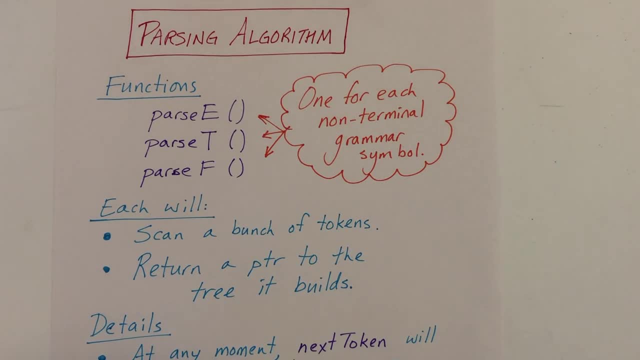 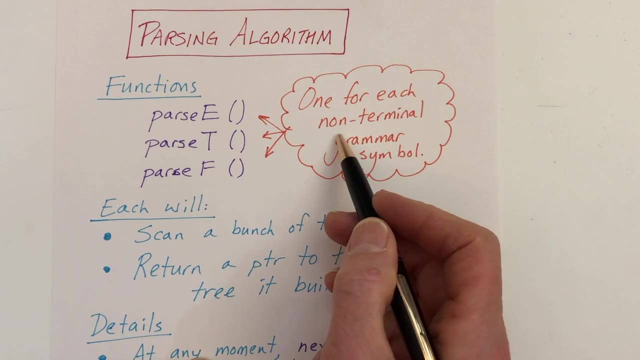 return it. We're now ready to describe the top-down recursive descent parsing algorithm. We're going to have a bunch of functions, one for each non-terminal grammar symbol. Each of these functions will scan a bunch of tokens and will return a pointer to the tree that 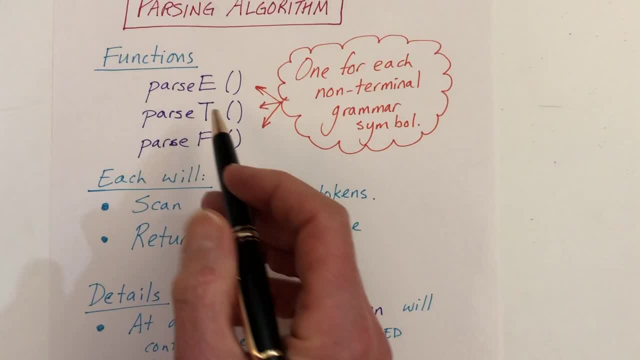 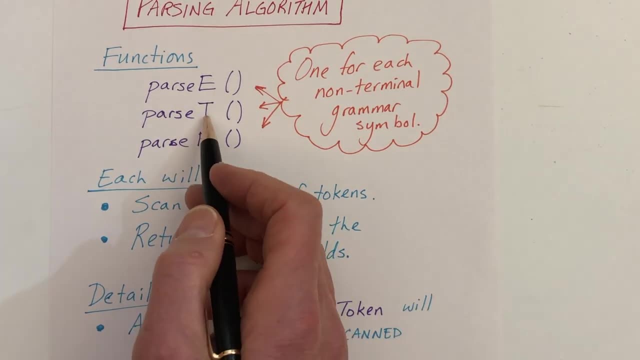 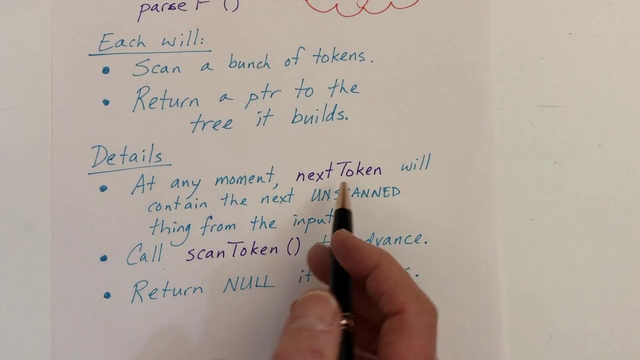 it builds to represent whatever it parsed. So, for example, parseE will parse an expression and return a pointer to the tree for that expression, parseT will parse a term and parseF will parse a factor. At any moment we'll have a variable called nextToken, which will contain the next unscanned 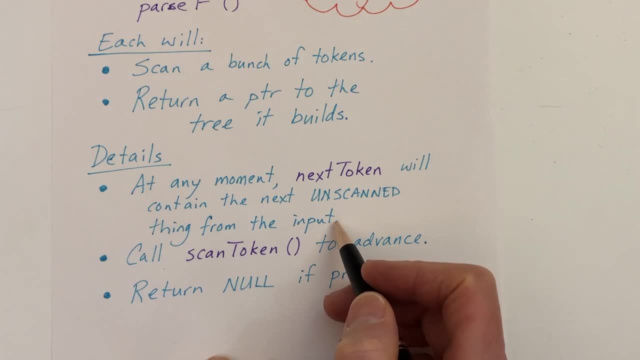 token from the input so we can look at it and see what's coming up. We'll call our lexer function scanToken to advance to the next token, that is, to read in some more input and see what the next token in the input stream is. 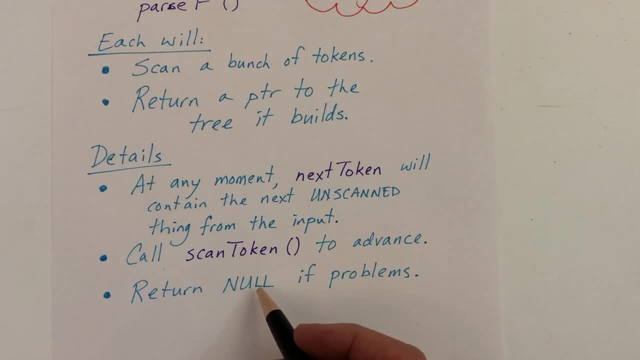 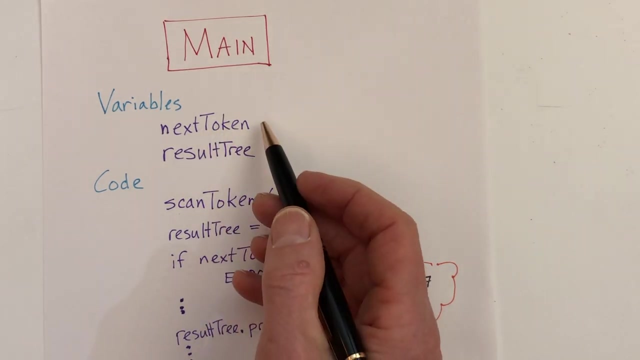 If there are any problems- and by problem I mean the input is not grammatically correct- then these functions will return null. So here's the overall organization of the program. We'll have a couple of variables. nextToken is a global variable that's shared among all the parsing functions, and we have a variable. 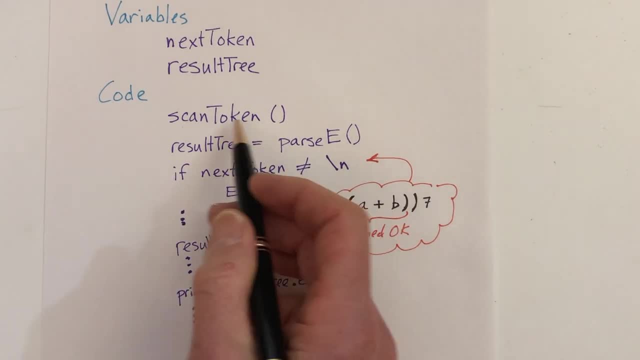 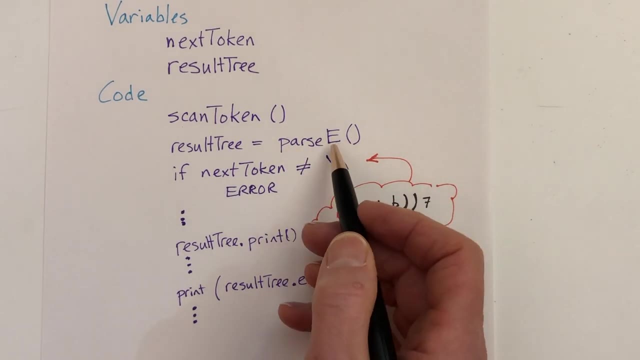 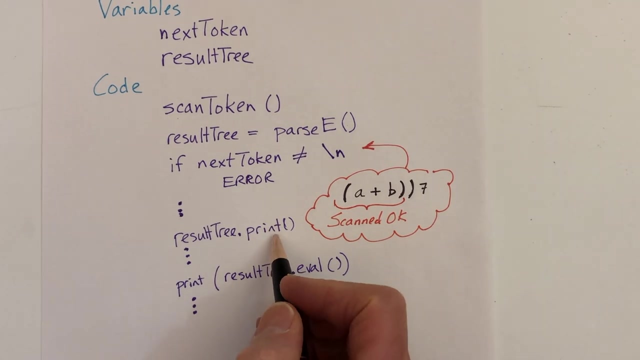 called resultTree. So what our program is going to do is start by scanning the first token and then calling parseT, parseE to parse the entire expression. That builds a representation which it returns, and we store that in resultTree. Then we might print out that tree to see what it is we read in: 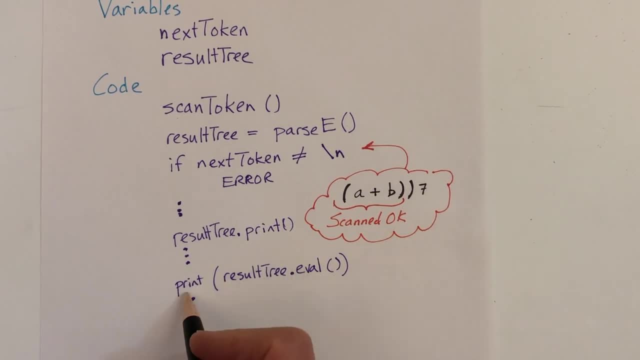 or we might call eval to evaluate the expression and then print the result. After we parse the expression, we need to make sure that the next thing on the input is the new line or the end of file or the end of input. Otherwise it's an error because we could. 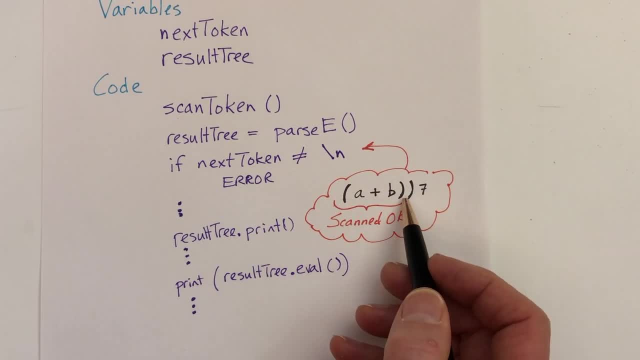 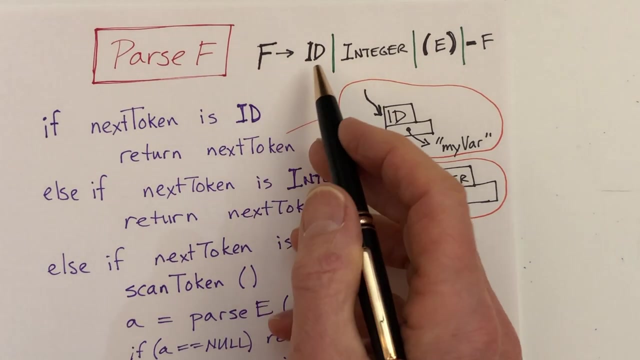 have some kind of input like this. Here we can scan an expression properly- no problem there- but we need to make sure that the next thing is not anything else besides the end marker. Let's look at the function that parses a factor which can be an identifier. 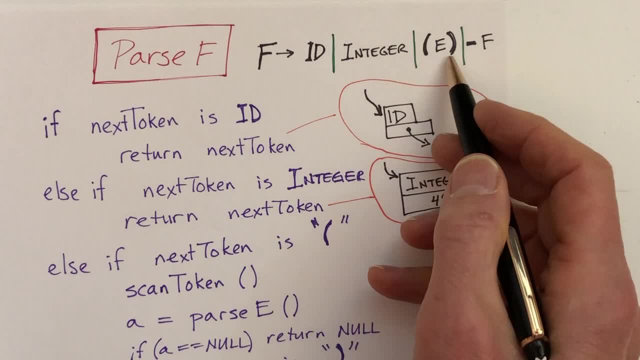 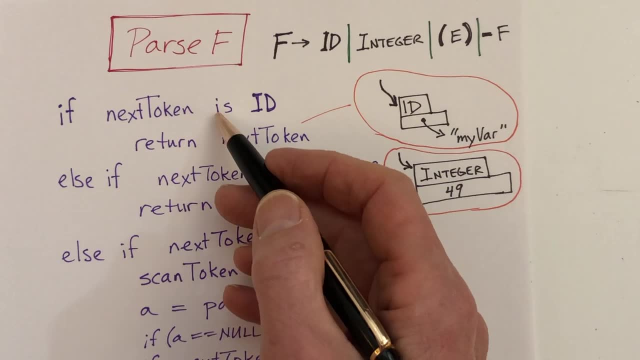 an integer or an expression inside parentheses or a negation symbol followed by another factor. So the function is basically just an if statement. We check the next token to see whether it's an identifier, an integer, an opening parenthesis or a negation. 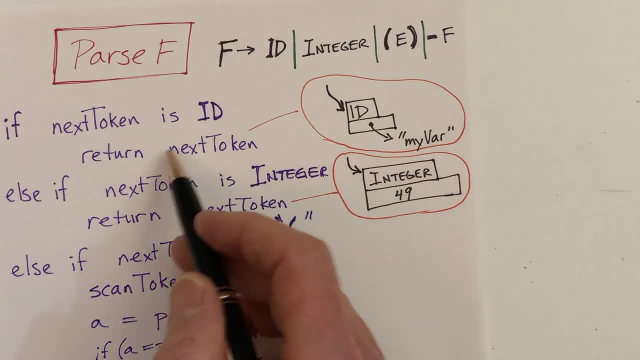 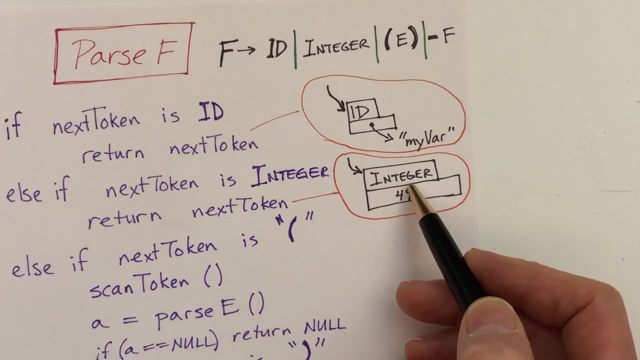 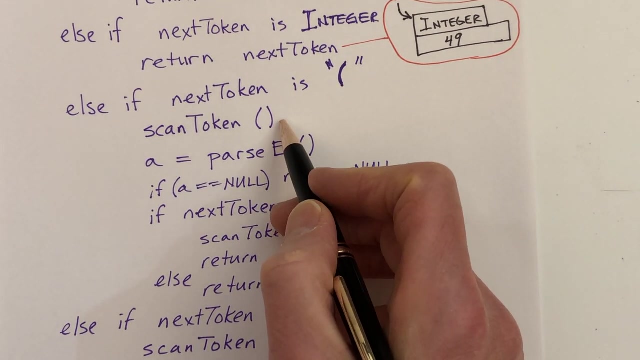 sign. If it's an identifier or an integer, then we simply return the token itself. More precisely, we return the object that represents the identifier or the integer. If the next token is an opening parenthesis, then we scan past that opening parenthesis to the next symbol and then we call parseE to parse an expression. Call it a, We can check to. 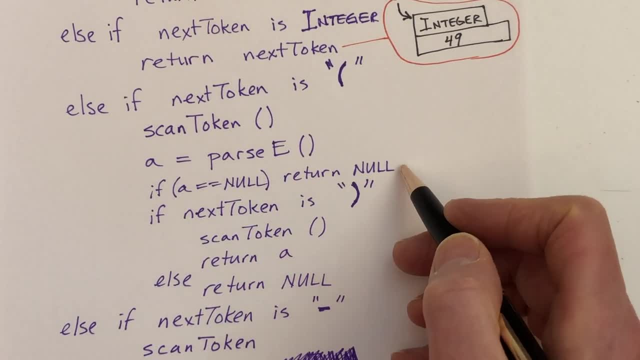 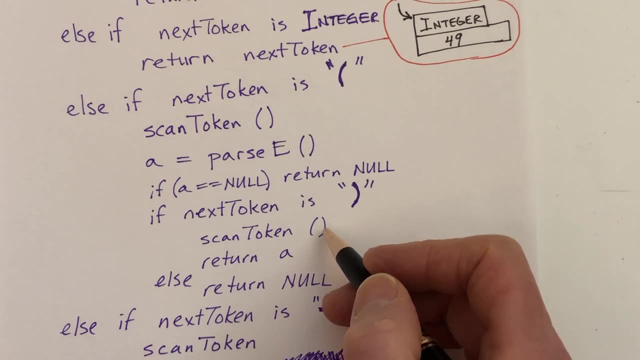 see whether there was an error and if so we just return null. And then we make sure that the thing following the expression is a closing parenthesis and we pick that up and finally we return the expression. If it wasn't a closing parenthesis, then we've got an error, so we return. 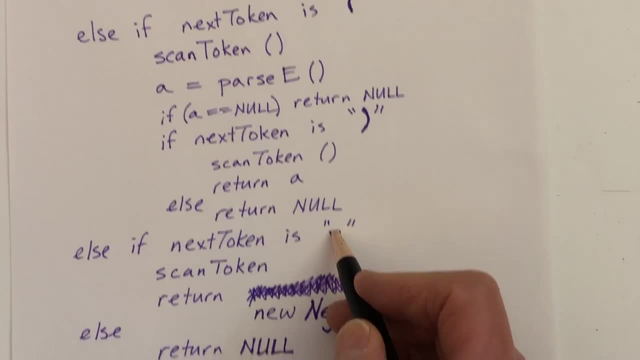 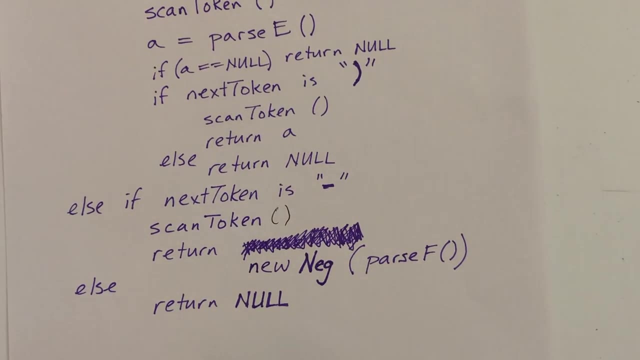 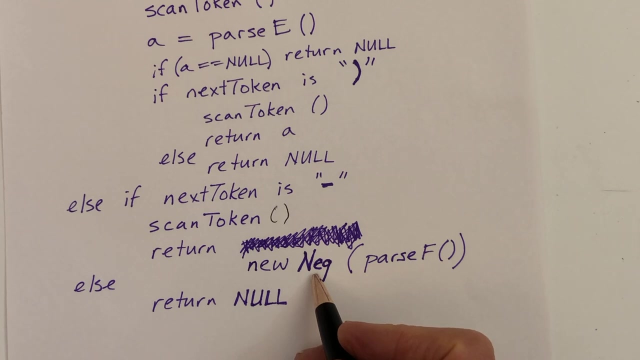 null. Finally, if we saw a negation sign, then we pick it up, we scan it- oh, I should put parentheses there- and then we call parseFactor To pick up another factor, and then we build a new object. Here we're saying new and we build. 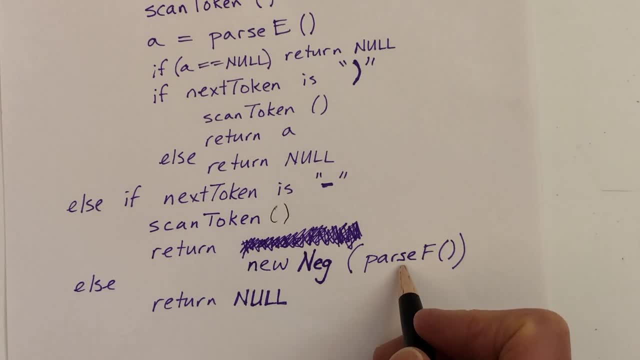 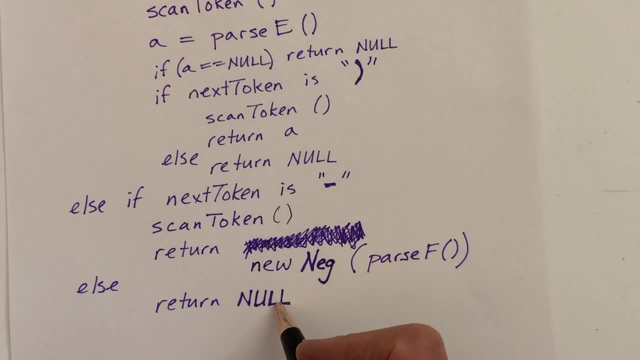 a negate object, whose argument will point to the factor that we just parsed, And if it's none of those things, then we return null. It was an error. Let's keep going with the function that parses expressions Before we go any further. 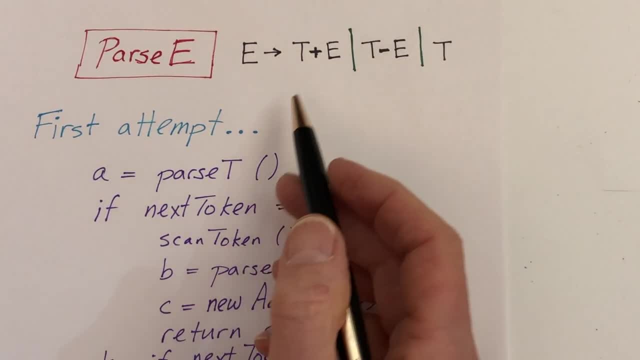 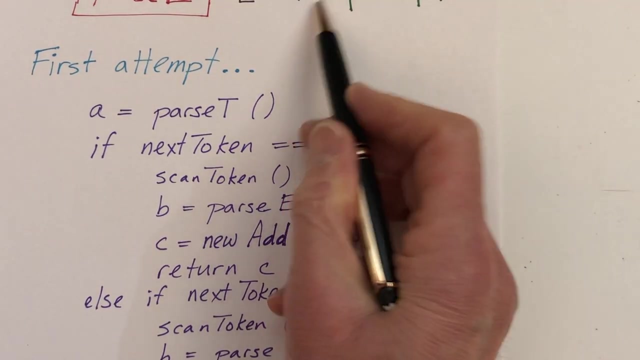 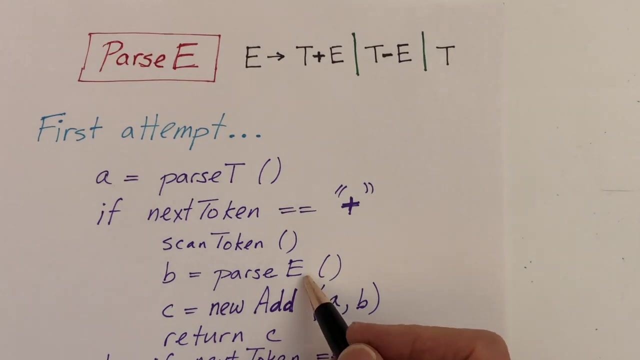 let me say that there's a problem with this code and I'll talk about that in a second. So an expression is t, c Lives an Jgergen. we're looking at something called the C weather. goodbye code. page 12: Lights Working- JGrefI emul. And then we start all three of these cases by picking up a term, so we call parseterm, And then we see whether we've got a plus or a minus. We've got a plus, then we pick that up, and then we pick up the e, that's calling parseE, right here. Then we build an add node using the first term that we parsed, followed by the expression b, and then we return null. and then we build an addEazi node using the first term that we parsed, followed by the expression b, and then we return null. 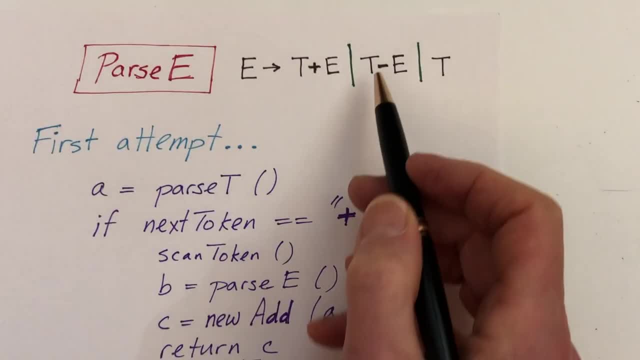 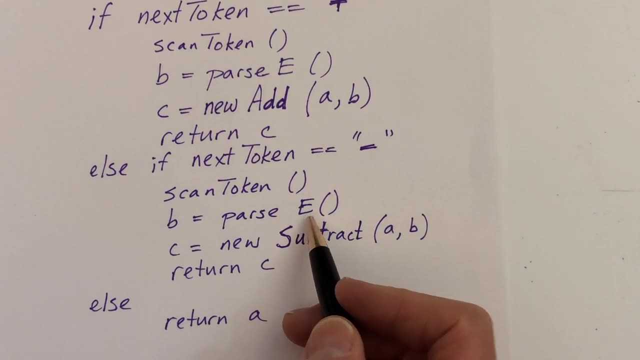 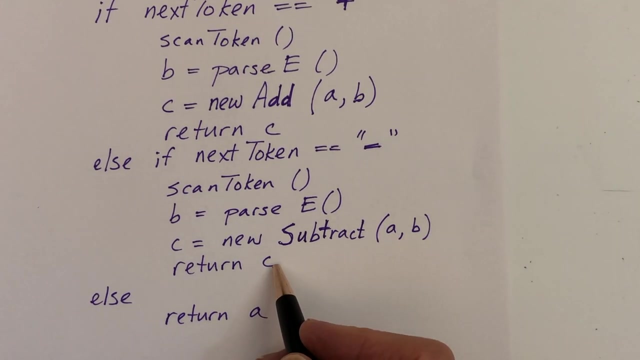 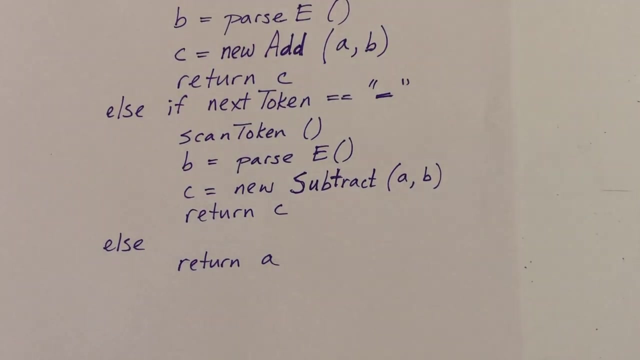 that node. If we have a negative sign instead, then same thing: we scan the negative sign, parse an expression and then we build a new subtract node with those two things and then we return that. And finally, if there's not a plus or minus following the T, then we simply return the term itself. As I said, the. 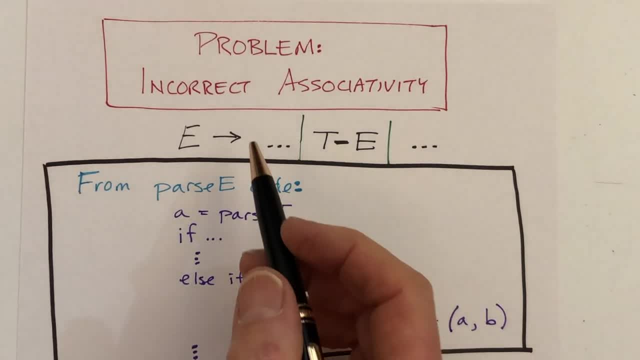 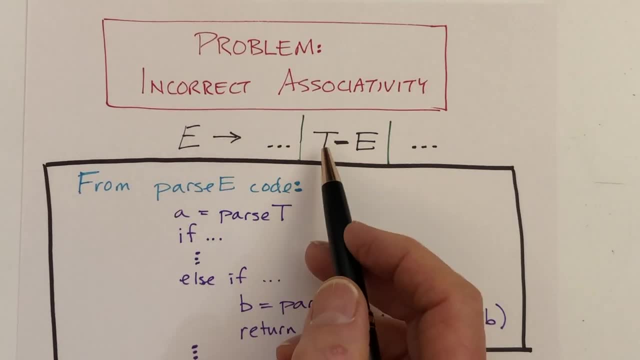 function as I just presented. it has a problem. It doesn't handle associativity correctly. To see it fail. let's look at this particular example. An expression goes to a term minus an expression. Okay, so the the relevant code. we pick up the. 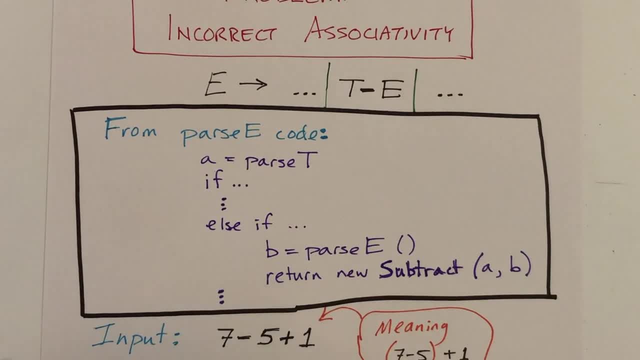 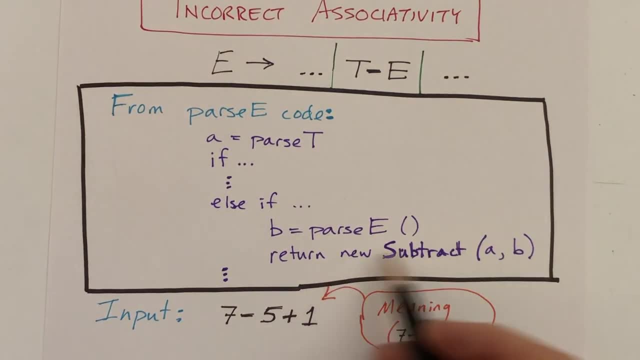 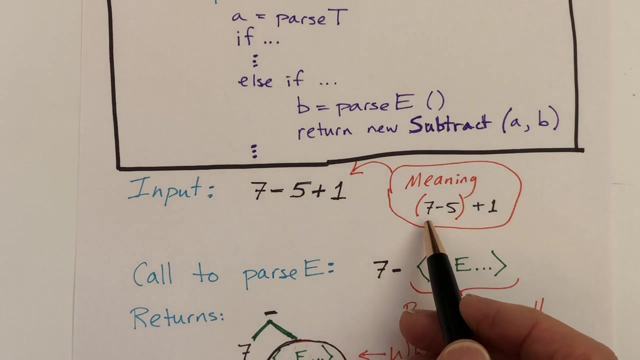 T by calling parseT. then we check and see we've got a minus sign. so we call parseE to pick up the expression and then we build a subtract node with the term and the expression. Let's look at this particular input: 7 minus 5 plus 1 and according to our rules of 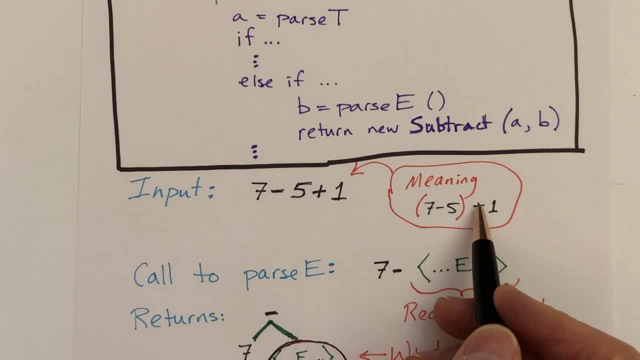 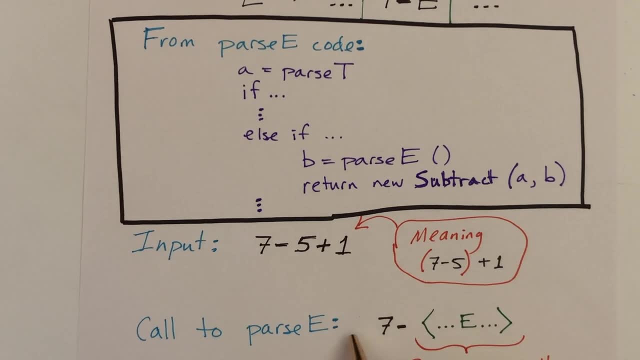 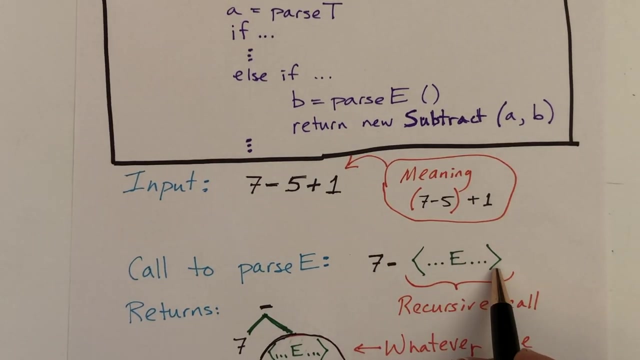 associativity. we do the subtraction first before the addition. So the way this thing will handle this expression is it first calls parseT to pick up the 7 and then it calls itself recursively to pick up another expression. So this call right here picks up the seven, then we see the minus sign. 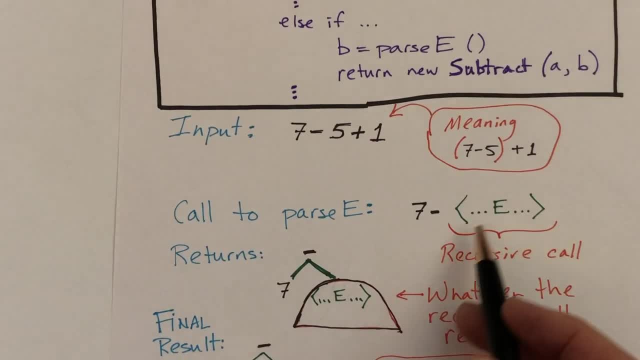 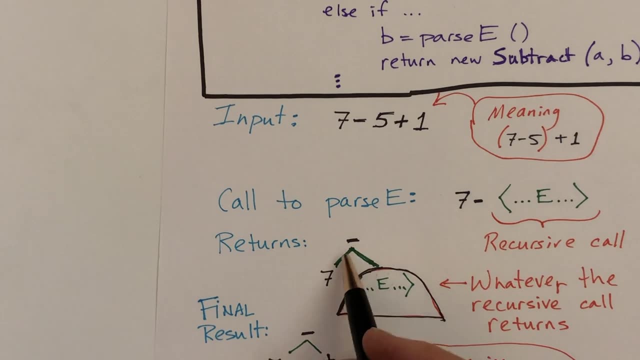 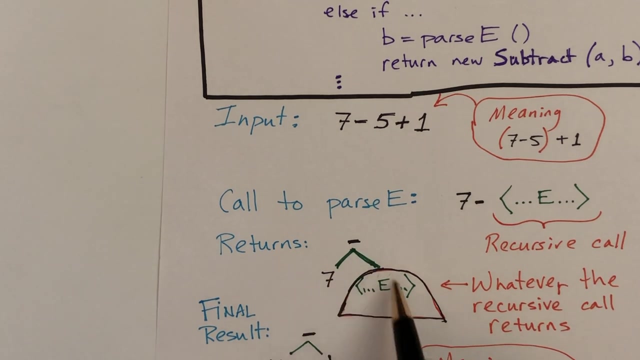 then we call parseE to pick up everything else, and so then it's going to build a subtract node with the seven and everything else that it picked up. So it's going to return a representation that looks like this tree here, minus sign at the root: 7 on the left and then everything else on the right. So 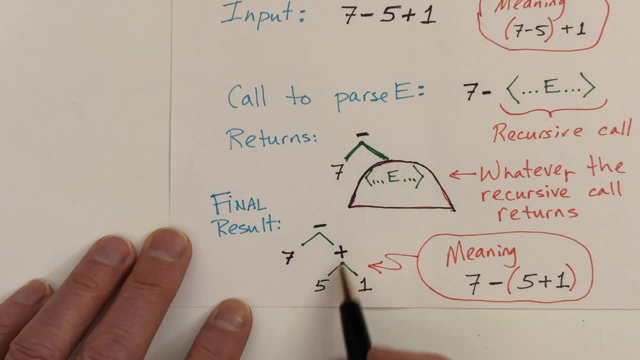 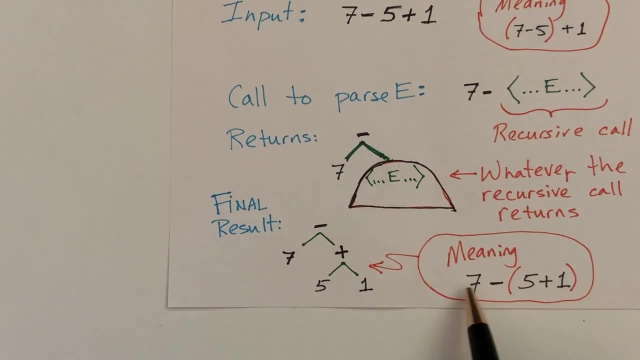 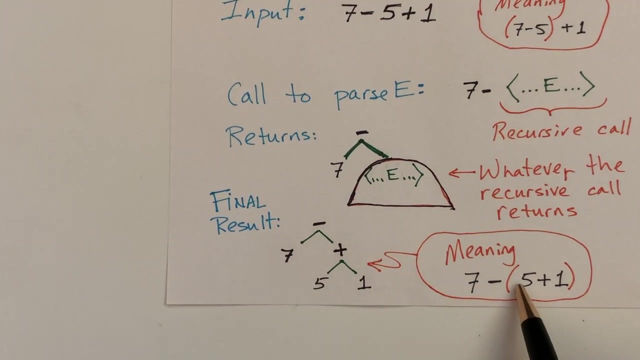 assuming that the rest of the expression is parsed, And that's 5 plus 1, so we have 5 plus 1 here and our final result will be this. But this tree has this meaning. It means take 7 and subtract the result of adding 5 plus 1, and that is not the correct. 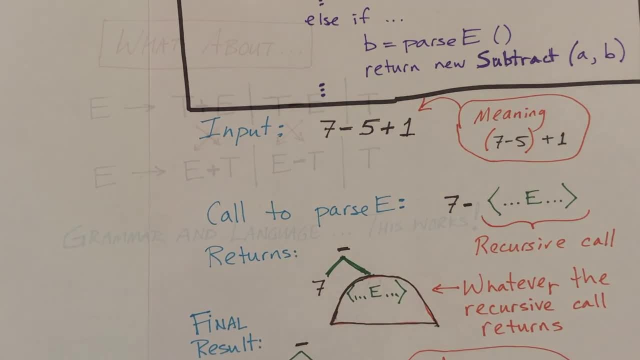 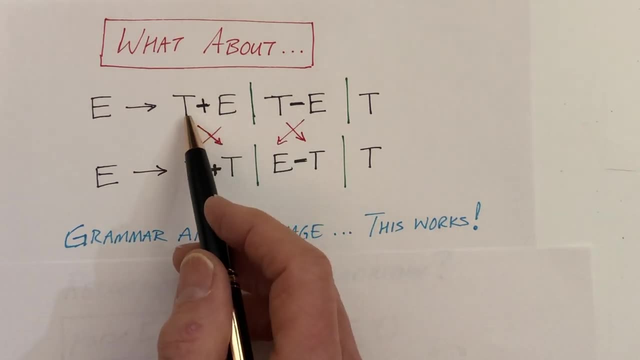 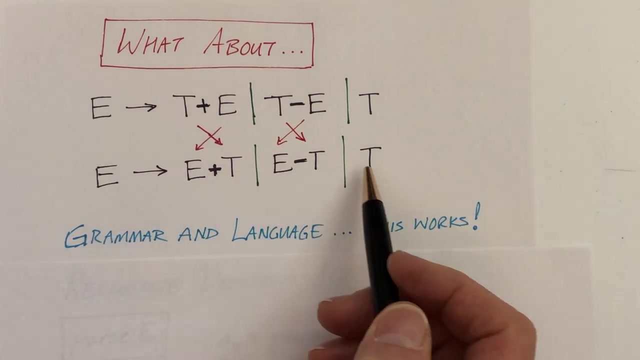 interpretation of our input. So now let's talk about how to fix this. We could always take our original rule and reverse the T and the E, So here we are producing a new rule with E plus T and E minus T, and that is a correct. 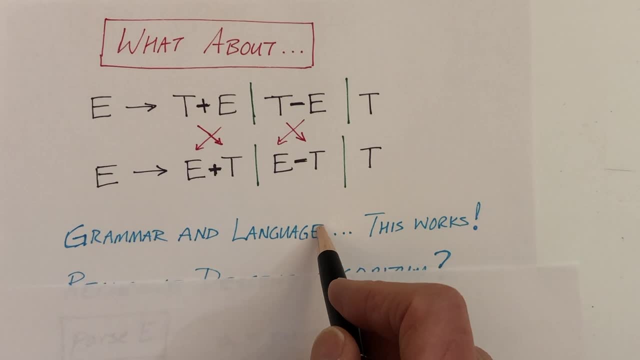 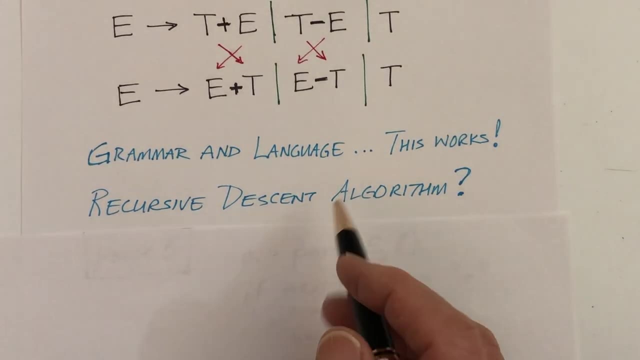 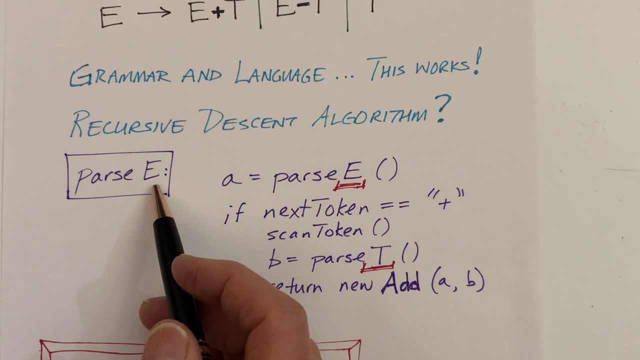 grammar and the language it describes is the same and, in fact, it models the associativity correctly. However, our recursive descent algorithm will not work with this particular grammar, So let's take a look at what happens. Here's our parseE function that we've now rewritten it using the second rule. 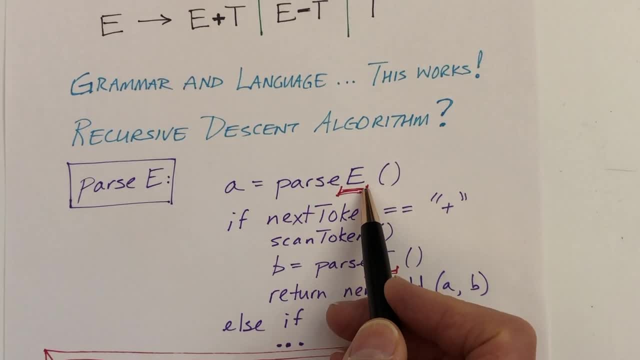 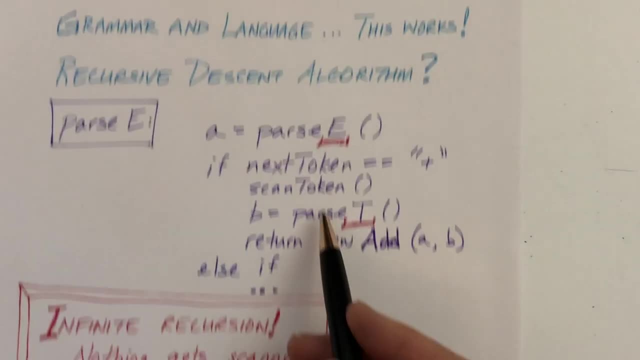 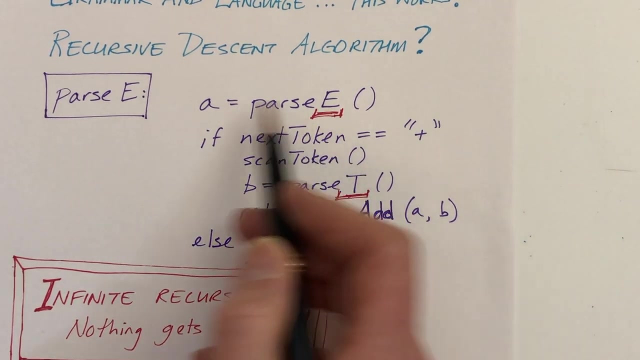 So the first thing we do is we parse an E- Okay, here we call parseE, and then we check the next token and if, for example, it is a plus, then we parse a T. So we scan the plus and we call parseT, and then we build a new add function using the result of parseE. 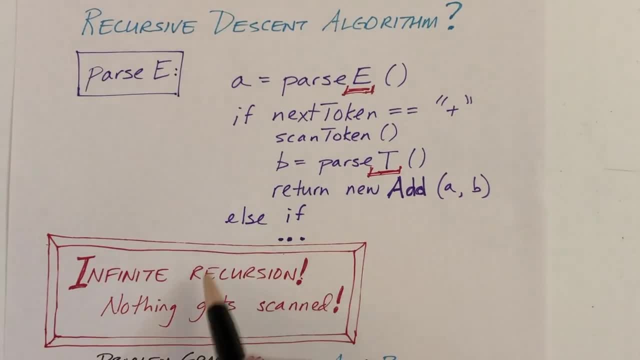 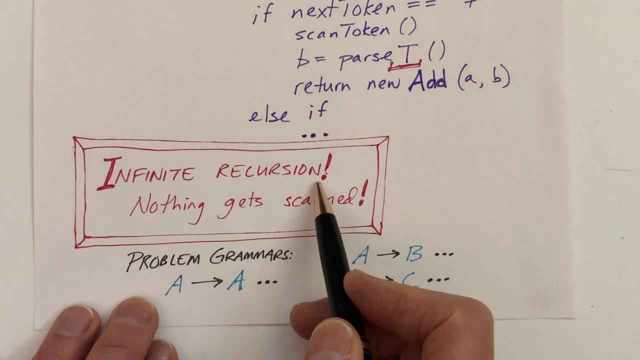 and the result of parseT A and B. However, this is infinite recursion. right, parseE? the first thing it does is call parseE itself without scanning any tokens. So this is infinite recursion. This is infinite recursion. nothing will ever get scanned, and this is a problem. 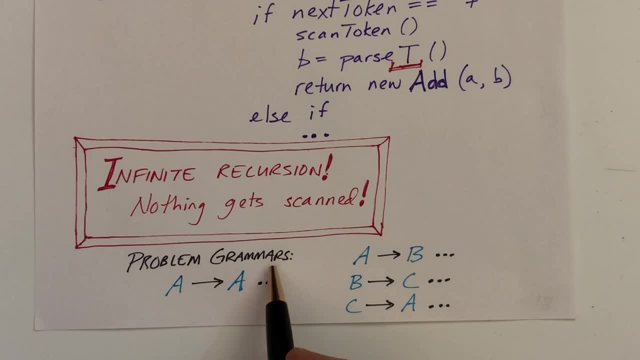 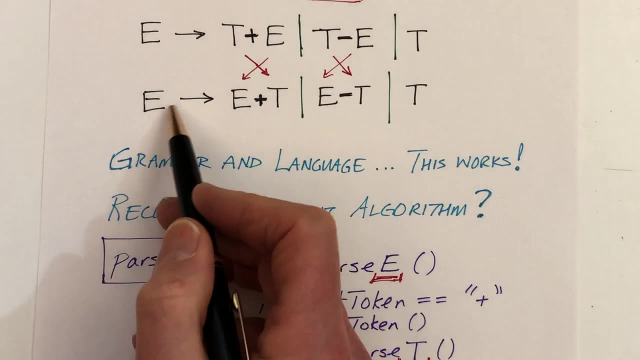 In general, the problem happens when we have rules like this in our grammar: A goes to something else and the right-hand side starts with the very same non-terminal. So we have that right here. E goes to E plus T. Okay. 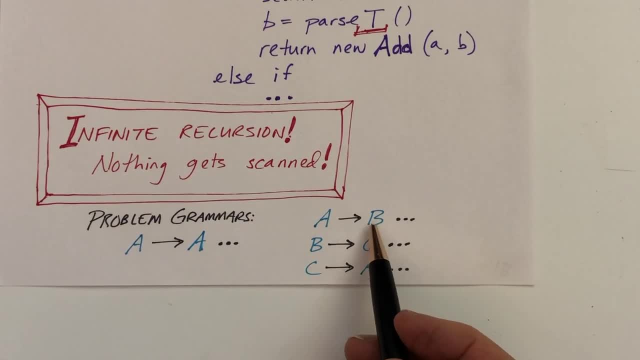 We can also have more complex situations. For example, A goes to a rule that starts with B, B goes to something that starts with T, Okay, It starts with a, C, and there's a rule for C that starts with A. So with grammars like this, we cannot use recursive descent parsing. 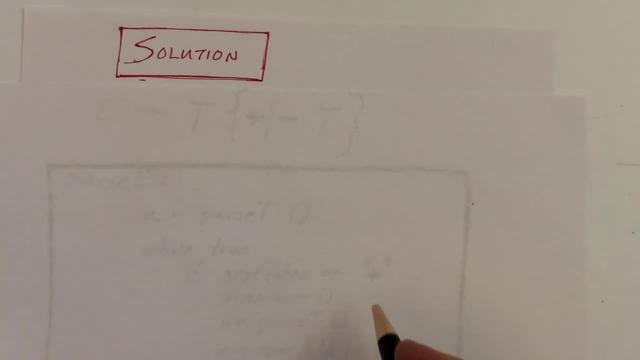 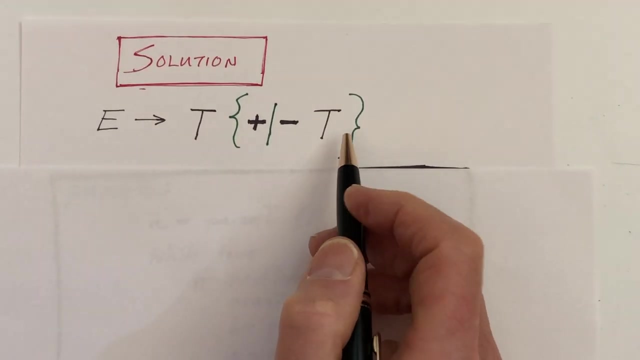 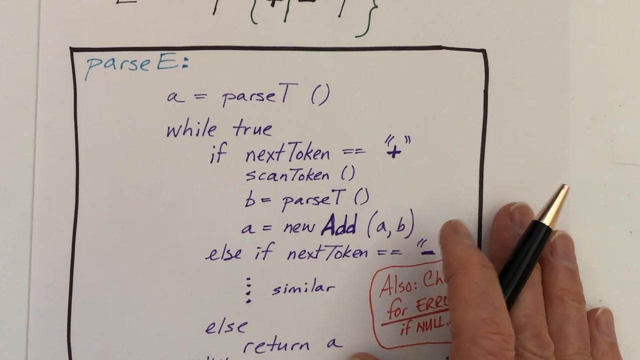 Fortunately, there's a nice, simple solution. What we're going to do is rewrite this rule as E goes to T, followed by zero or more occurrences of plus T minus T, plus T minus T and so on. Here's what the code now looks like for the parseE function. 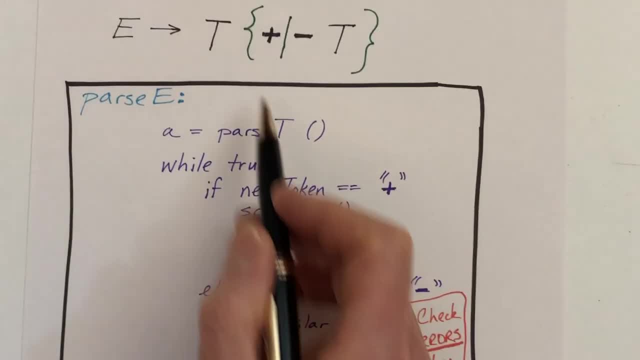 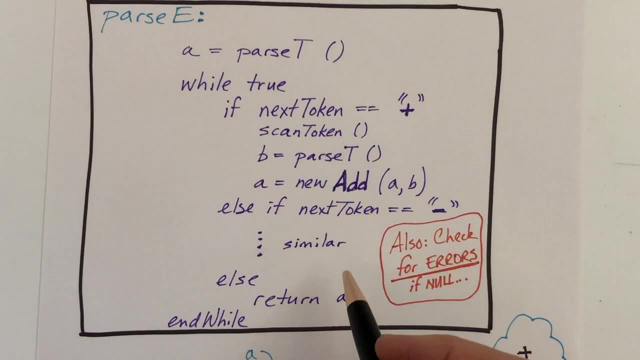 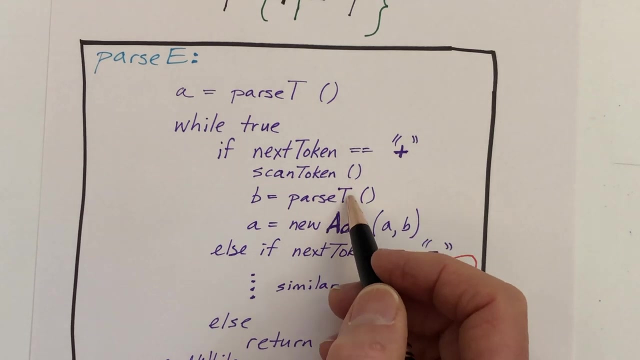 We first call parseT to pick up the first term and then we have a loop. So this is an infinite loop with a breaking. by returning We look at the next token. If it's a plus, then we scan it, and then we parse another T and we build an add node. 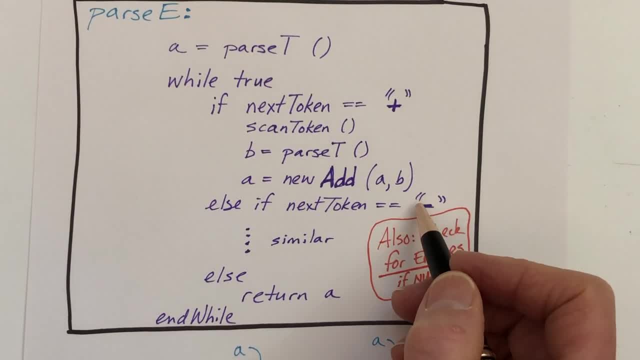 and we keep going. If it's a minus, we do a similar thing. If there's no plus or no minus, then finally we return A. So we're building up A all the while. I've left out the error checking code here, but you could figure that out. 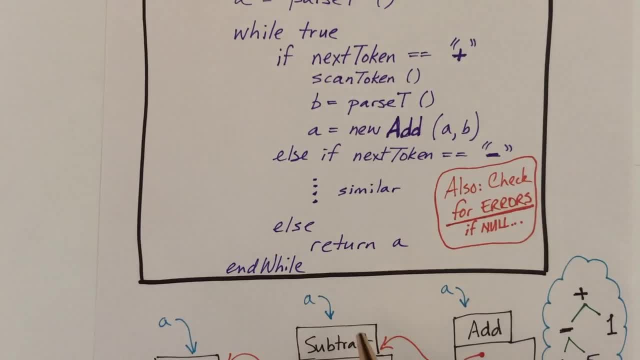 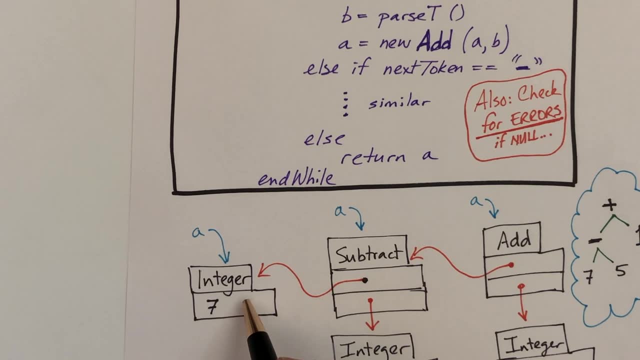 It's pretty straightforward: We just check for null. So let's see how this thing works on a particular example, We're parsing our seven minus five plus one. So we start by calling parseT and we pick up the seven. Okay, 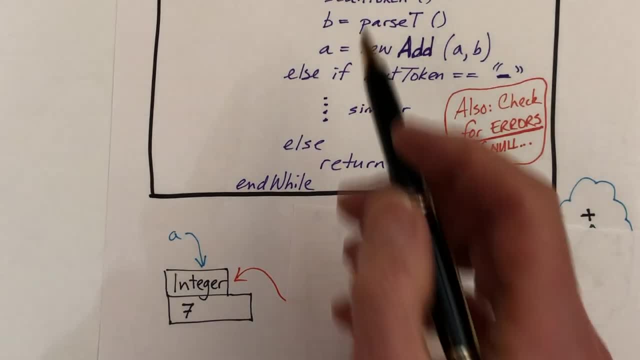 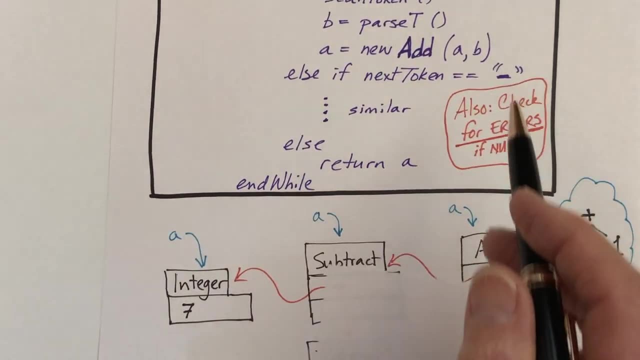 So that's what we get here At this point. we've parsed the seven and we've got zero. We've got A pointing to a seven. We go into our loop here and we see that there is a minus sign. So what we're going to do is scan the minus sign. 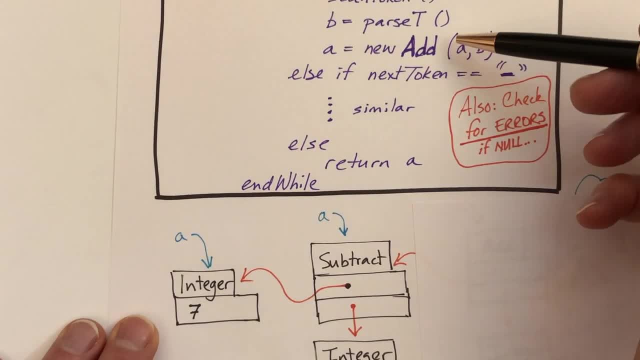 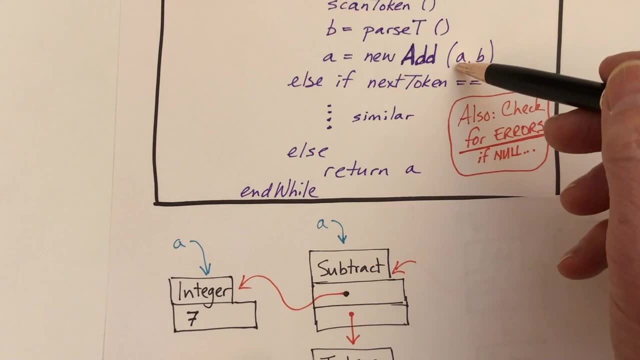 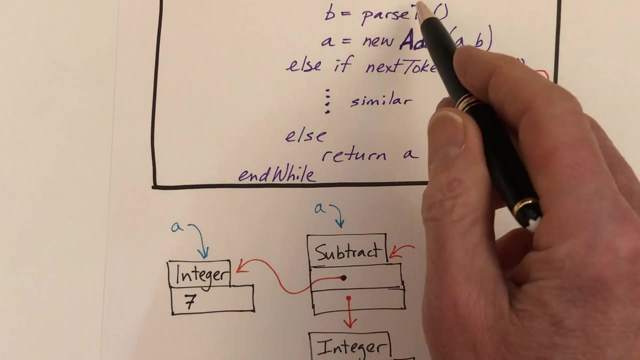 We're going to call parseT, and then we're going to create a new node, a subtract node, and we'll call it A. We're going to use as the left pointer the pointer to the previous A, That is, the pointer to the seven node, and B, the new node. 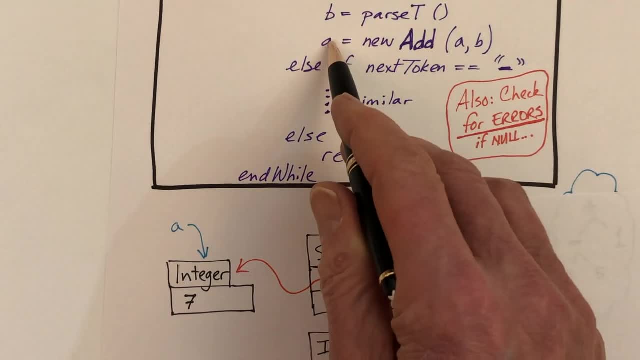 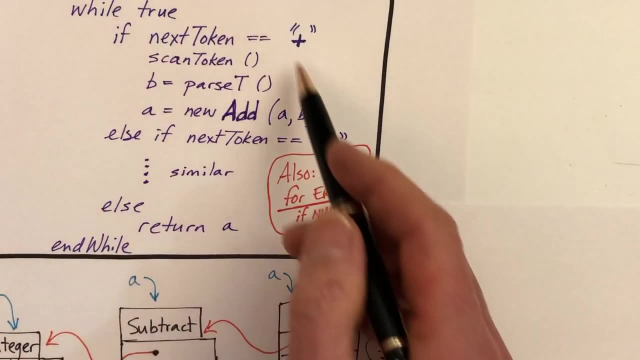 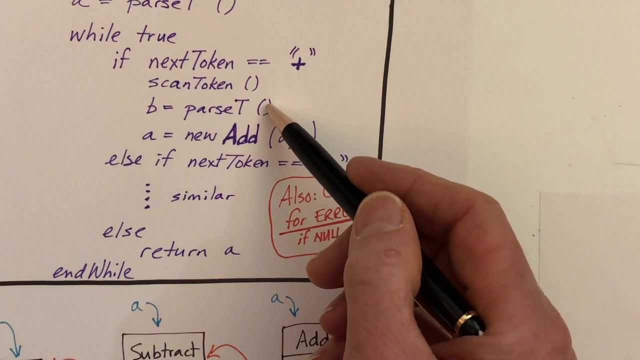 That's the term that we just picked up, which is five, And that will become our new A. Okay, And then we repeat the loop and what happens? We see that the next symbol is a plus sign. So we scan the plus sign and call parseT. 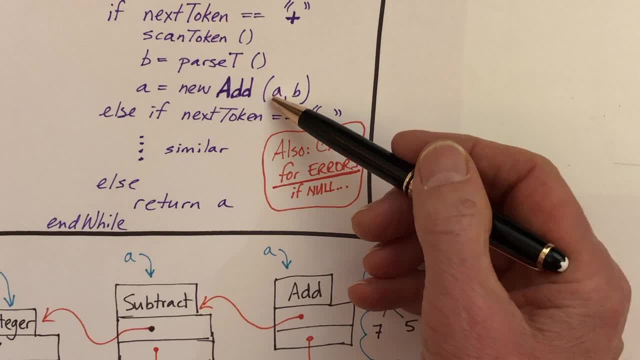 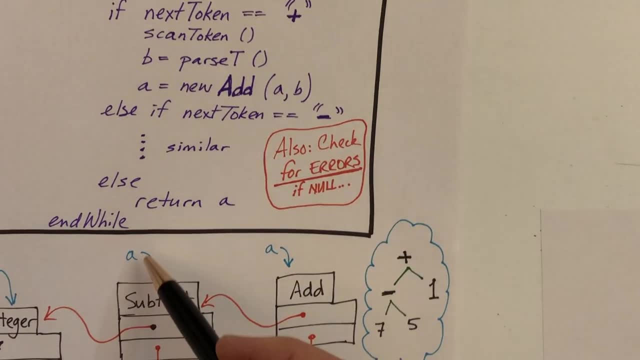 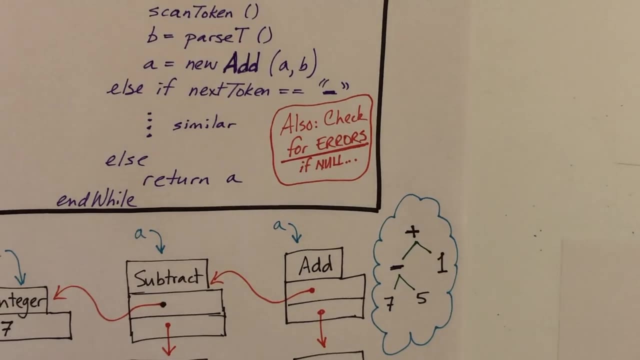 And here we pick up the one and we create a new add node using the old previous tree A. Okay, So we've got our new node, We've got the previous tree right here and the new one that we just picked up, the integer. 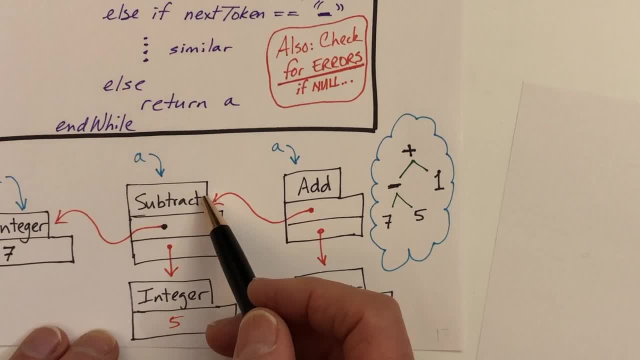 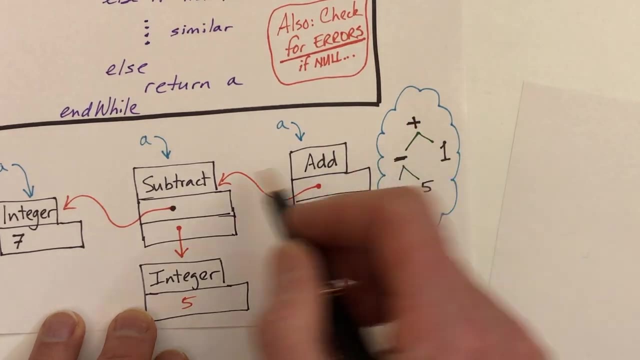 one. So here we build our new node. Our left pointer goes to the previous version of A and our right pointer goes to the integer one. So this is a tree. It's not written very much like a tree, So if I reorganize it, you can see that the top node is an add. 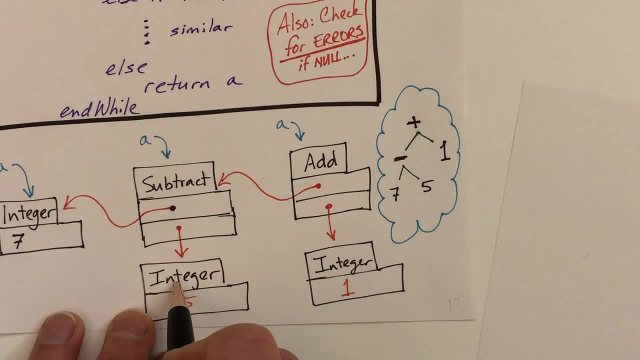 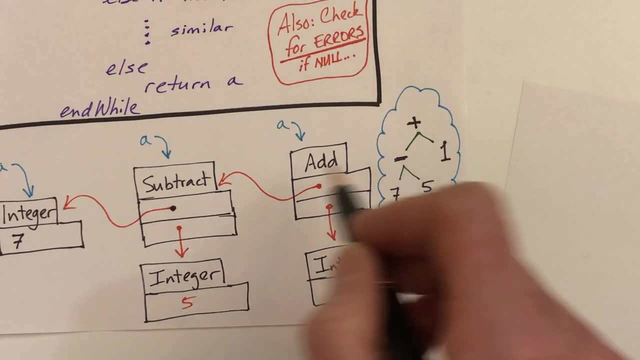 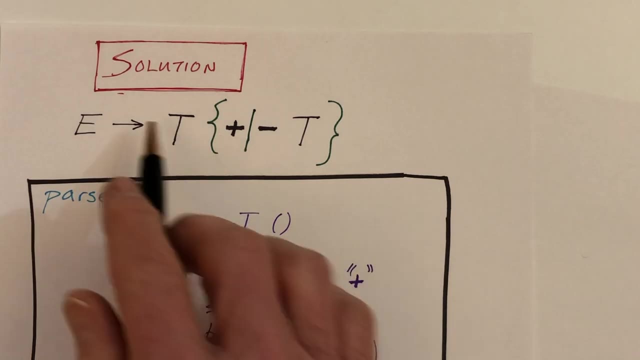 Left goes to a subtract and then it's subtract seven minus five And the other operand to the Addition is one. So it is this interpretation that this code will build up. The rule for T is similar. We have to modify it in a similar way because it has the same infinite recursion problem. 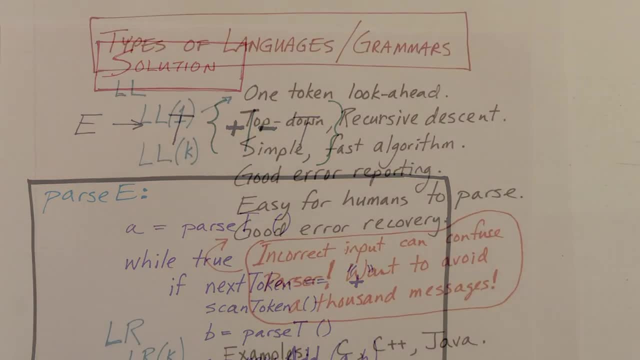 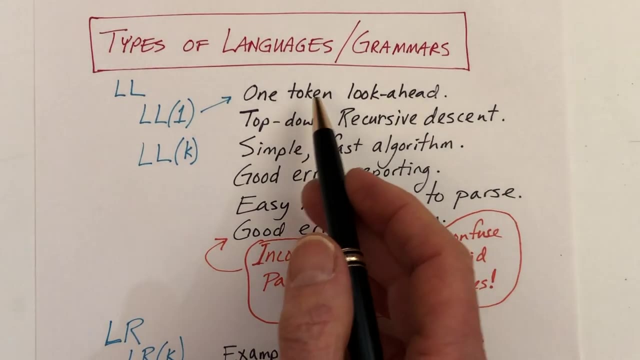 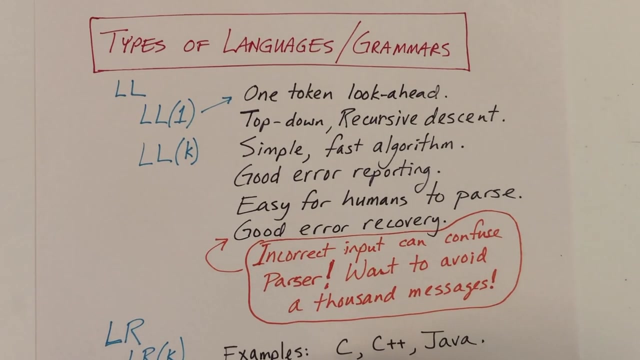 as it's written right now, But I think you can do that. I taught compiler design and theory of computation for several years and the whole subject of languages and grammars and parsing algorithms is really quite fascinating. There's really a lot to it. 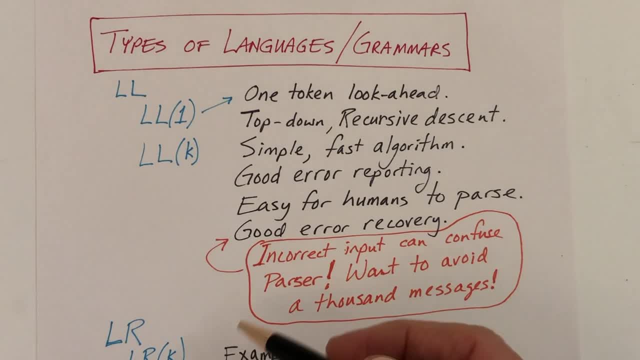 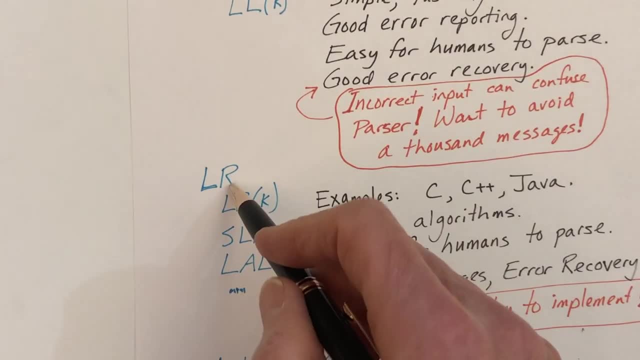 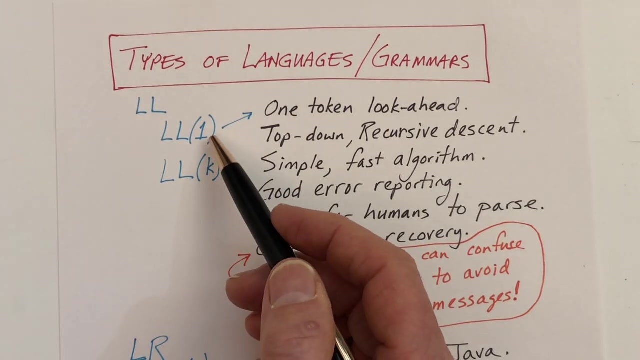 Basically, we can break down languages and parsing into several different categories. We have LL languages, LL parsers, LR and everything else. We've been talking about something called LL1.. Our grammar is LL1.. That stands for the one is for one token, look ahead. 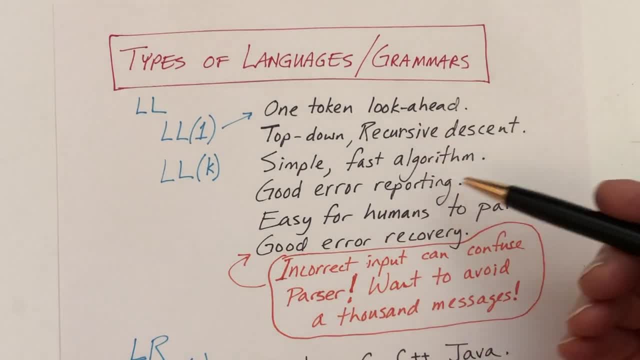 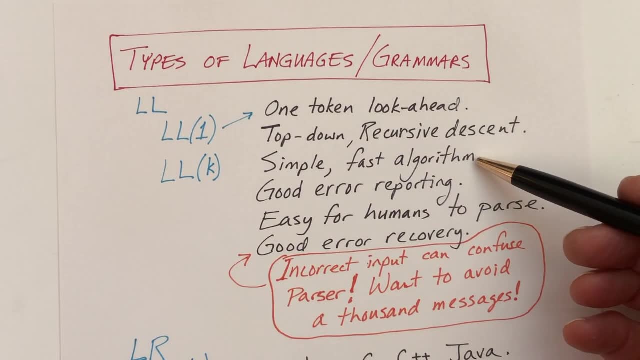 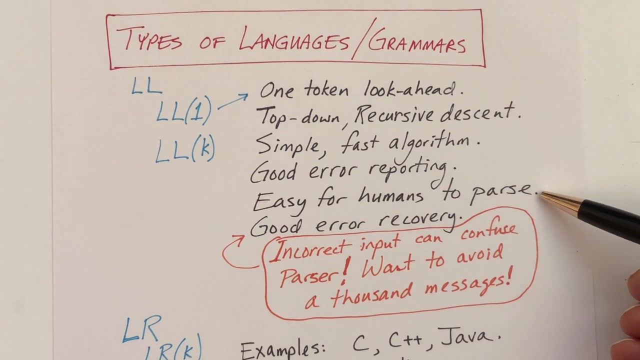 So we can basically see where we're going just by looking at the next token. It's great because we can create top-down recursive descent parsers. That's a very fast and simple algorithm with good error reporting, And these languages- LL1 languages- are very easy for humans to parse. 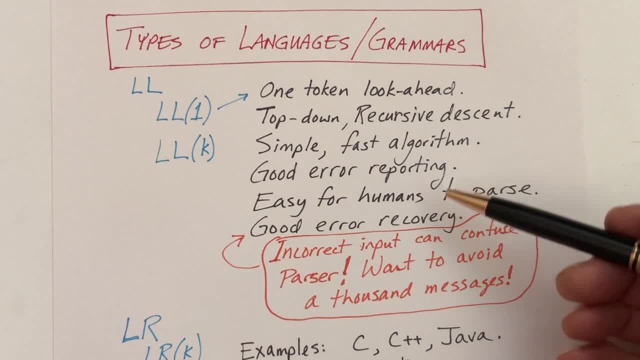 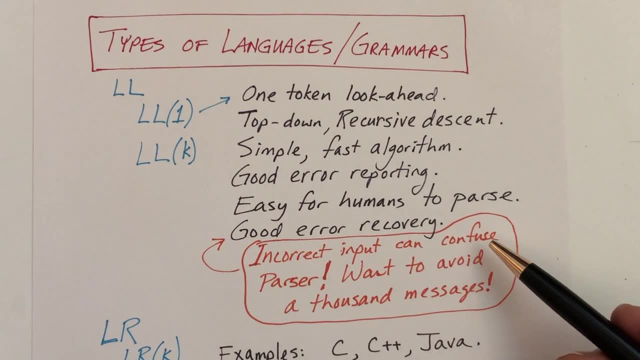 And another thing that's important is we have good error reporting and good error recovery. The user often will have incorrect input and that can really confuse a parser. We want to avoid printing out a thousand. We want to avoid printing out a thousand. 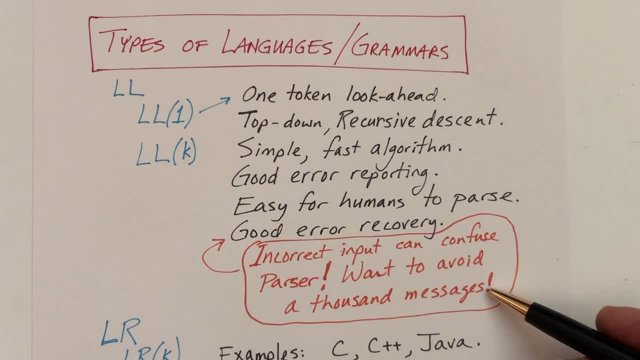 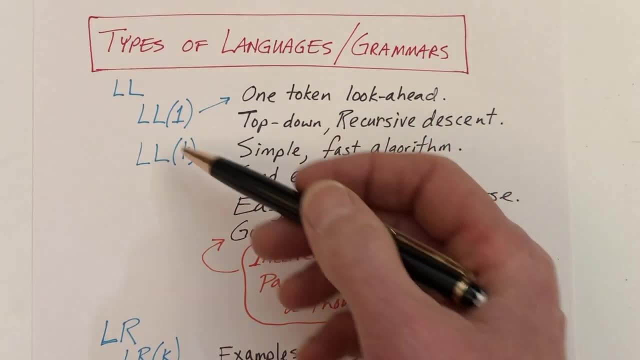 We want to avoid printing out a thousand different messages from one single error. We want to print out a nice concise error that tells the user what they did wrong. There is a class of languages called LLK, and LL1 is the simplest version of that. 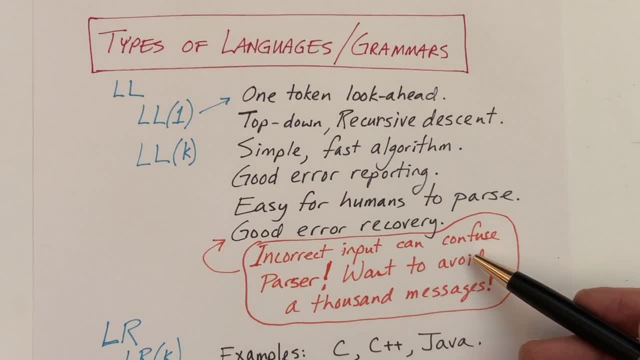 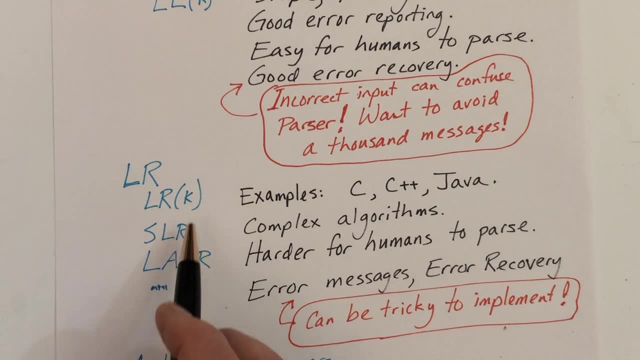 And, as I said, the grammar that I presented here is LL1.. We've also got more complex grammars and languages called LR, LRK. in general, There's some variations: SLR and LALR. I'm not going to go into what all these stand for, but these are necessary for more complex programming languages like C and C++ and Java. 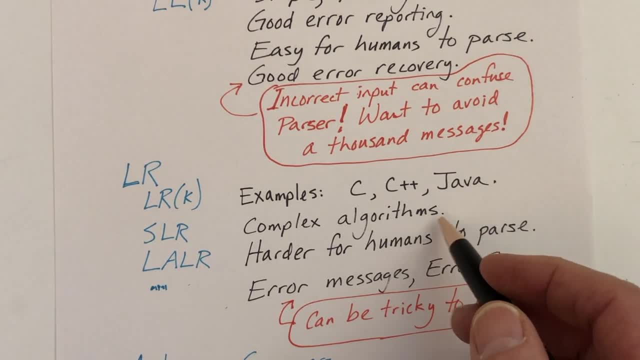 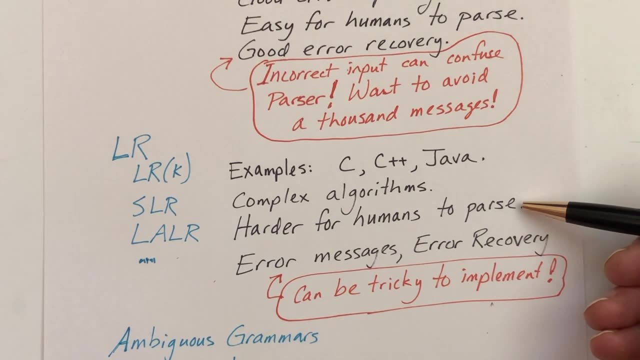 The algorithms for parsing are more complicated. In fact they're really quite complicated. I've taught them for many years and it's really hard for the students to understand. Hard for me to understand at first, in fact. These languages are also harder for humans to parse. 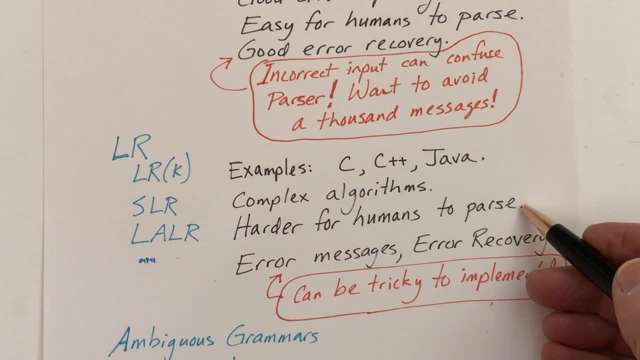 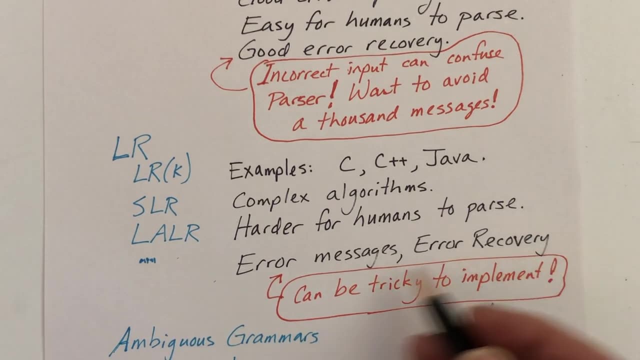 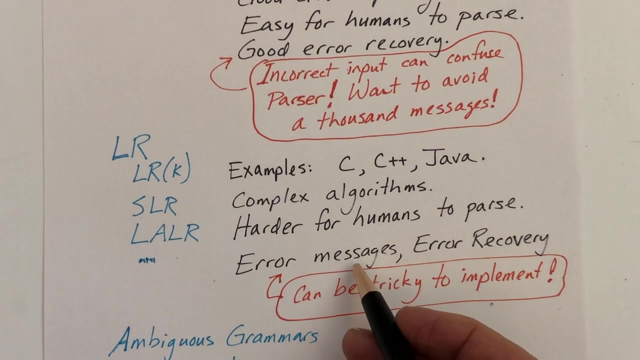 And I think that's really very relevant. I don't want a complicated language particularly. Life is complicated enough without the unnecessary complexity of languages. These languages also are more difficult to create parsers that produce good error messages and recover appropriately from errors, So that's really a practical issue. 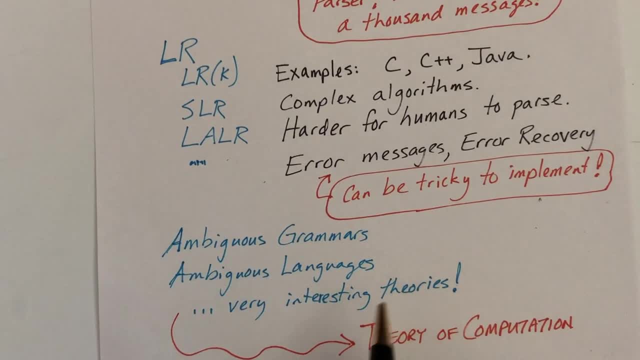 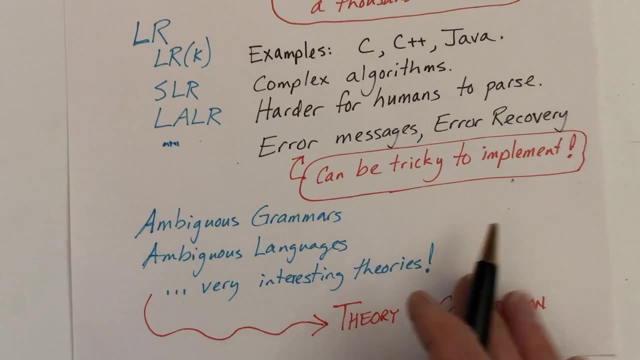 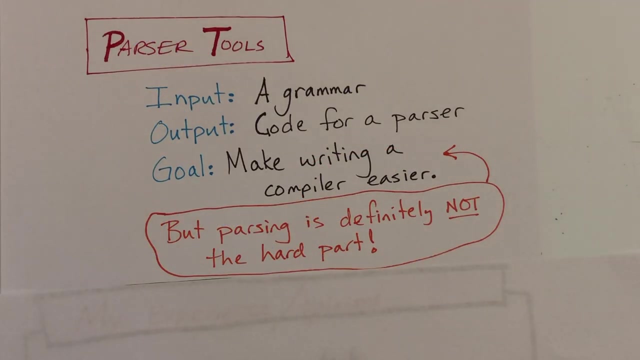 Beyond the LR and LL grammars, we have ambiguous grammars and ambiguous languages. It gets even more interesting after that and gradually goes into the theory of computation, But that's for another video. One thing you may have heard about is parser tools, also called parser generators. 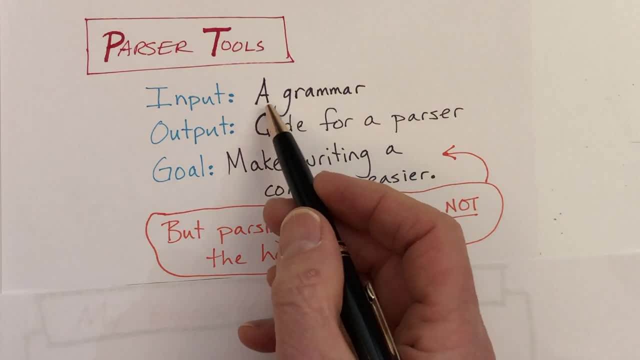 The idea with one of these tools is that the input is a grammar, So you're putting a grammar into the tool and the output is a parser, Or, more precisely, code for a parser Or something that you can embed in your own code. 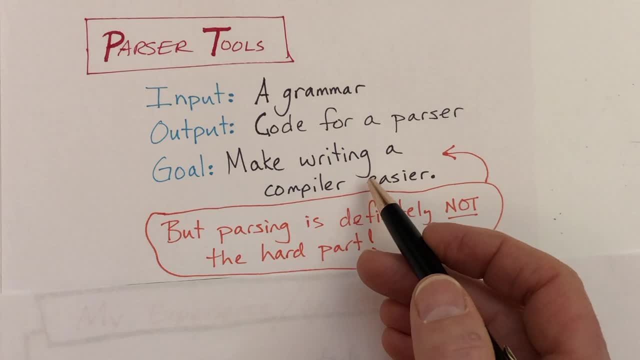 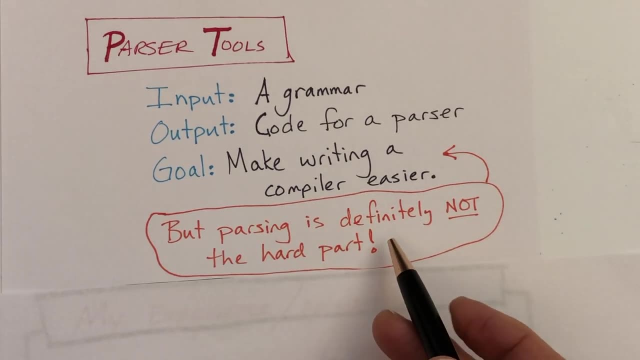 And the idea is that these tools are supposed to make writing a compiler easier. I do want to say that parsing is definitely not the hard part of writing a compiler. Having written several compilers, I've learned that the parsing is really the easiest part. 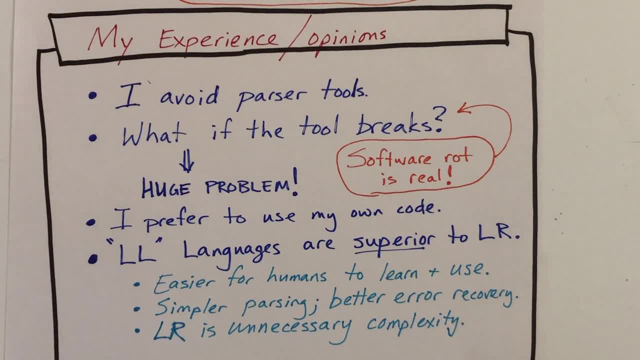 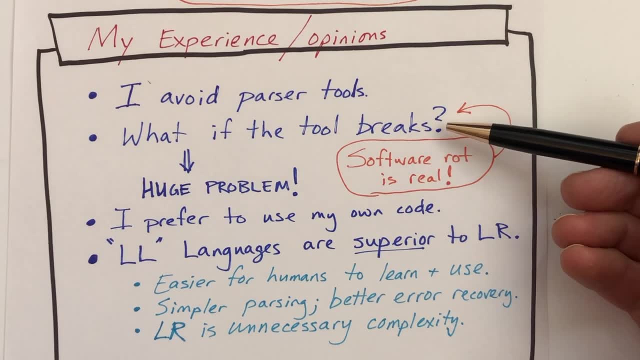 In fact, you know, my opinion is that I prefer to avoid parser tools altogether. You know the tool can break Software. rot is real. Things that used to work suddenly stop working because of upgrades in other software that they depend on. And it's complex.